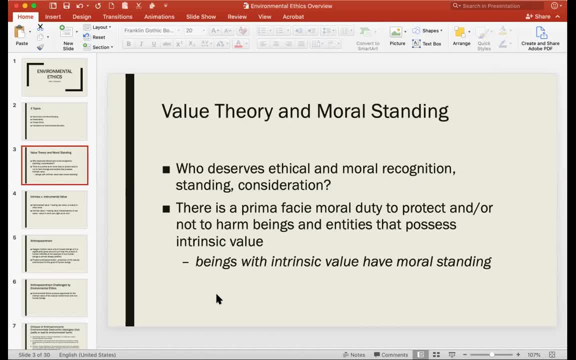 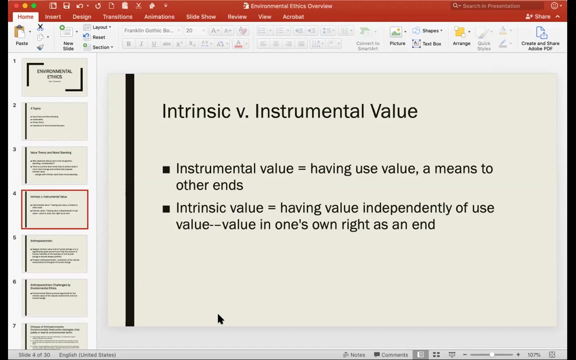 they are morally considerable. So how we conceive value, Whether a being has value, Intrinsic value, is foundational to our moral duties to them, And we can make the distinction between intrinsic and instrumental value. That instrumental value refers to having some kind of use, value being of use. 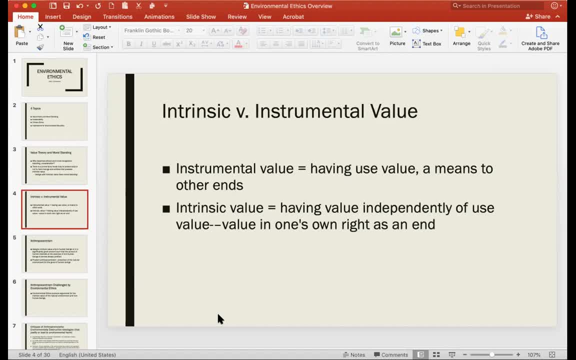 Things that have instrumental value are a means to other ends. Okay, We made ins and int values verbatim and we can use them to enhance instrumental. So inanimate objects like this computer that I'm using today has instrumental value. 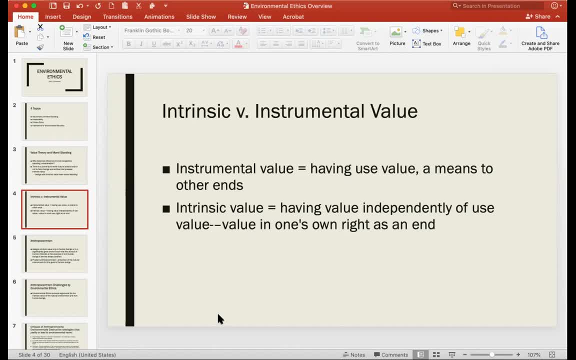 It's a means to other ends. It's a means to other ends. Intrinsic value refers to having value independently of of use value, And intrinsic value, therefore, is value in one's own right as an end, And it's very important to this in some way, just to make the Magnetoassette view. 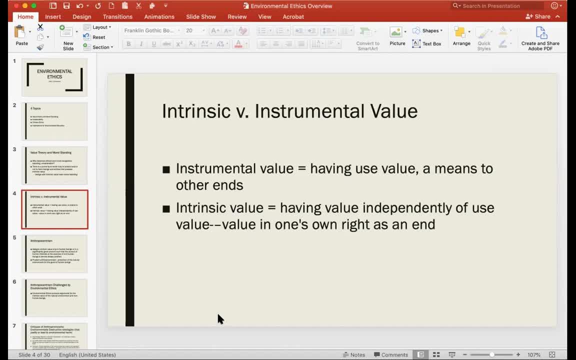 Matters, Matters, yeah, Matters. yeah, Name is value, And that would unconditionally be Mohammed and Sattler value for us as individuals and individuals. Yeah, Uh-huh, Network остав On, okay. So intrinsic value refers to beings who are subjects, who are ends in themselves and not merely means to other ends. 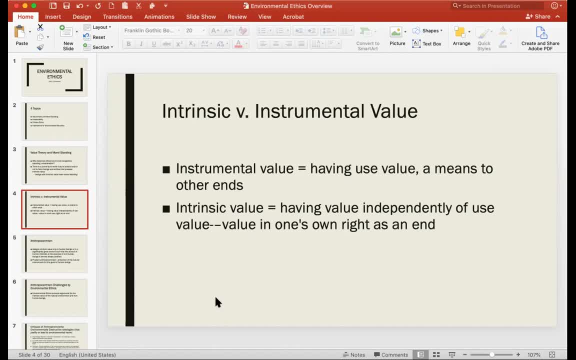 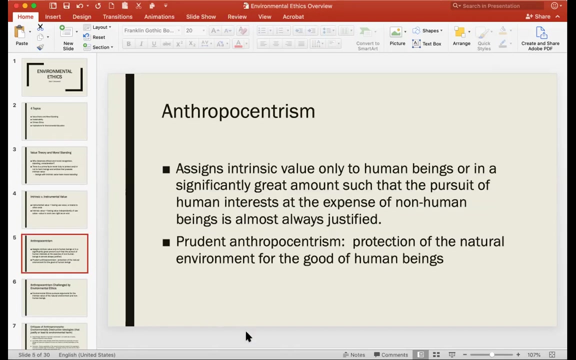 And one of our basic moral convictions is that human beings have possess an equal intrinsic value as ends. The question of environmental ethics is that: can we extend that notion of intrinsic value to non-human beings? Anthropocentrism assigns intrinsic value only to human beings, or in a significantly greater amount. 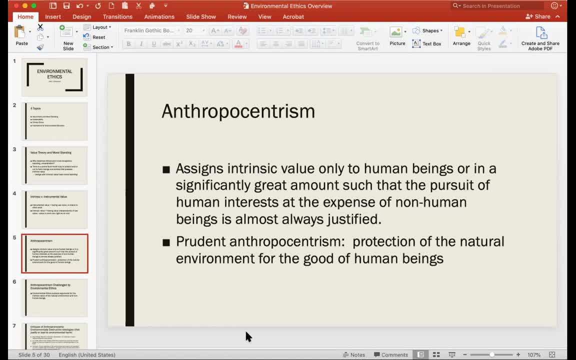 such that the pursuit of human interests are justified At the expense of non-human beings is always justified. So from an anthropocentric point of view, from a human centric point of view, other living beings only have instrumental value. We may develop an environmental ethic based upon anthropocentrism, in the sense of prudence that the protection of the natural environment 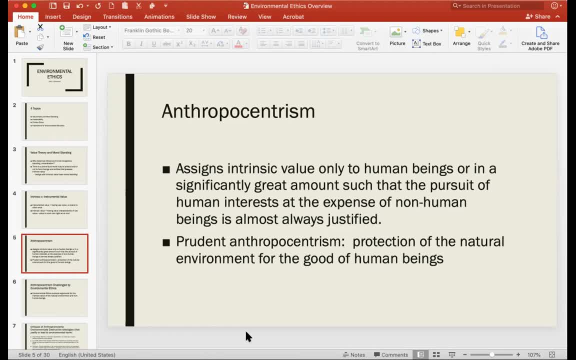 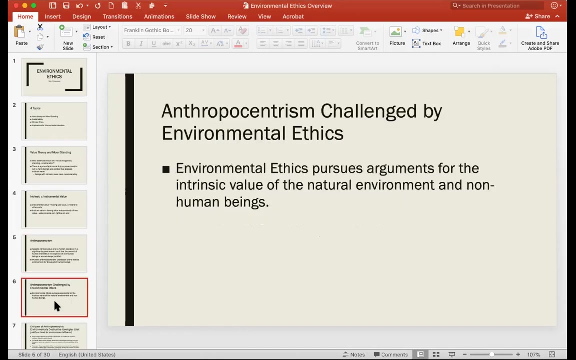 and the beings that inhabit that environment. that protection is good for human beings. And often environmental considerations are couched in this anthropocentric orientation. We view the environment and other living things as having instrumental value to the good of human beings. Much of anthropocentrism is challenged by human beings. 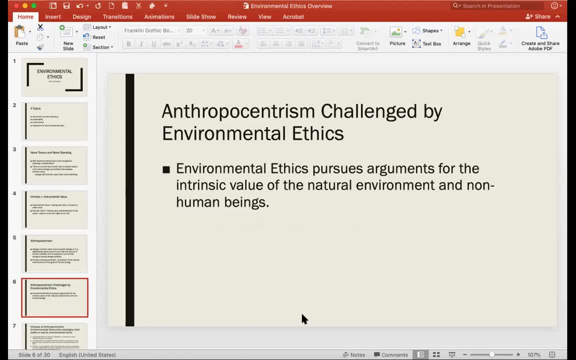 Much of anthropocentrism is challenged by human beings. Much of anthropocentrism is challenged by human beings. Our own approach to the United States is subject to structural environmental ethics, which pursues arguments for the intrinsic value of the environment and non human beings. 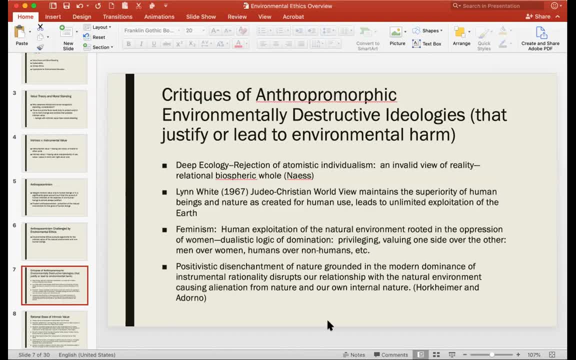 There have been a number of critiques of anthropomorphic or anthropocentric patterns of thought that may have been argued to be environmentally destructive, that may have been argued to be environmentally destructive, that justify or lead to environmental harm. and these are four noted critiques of anthropocentrism, the one coming from deep ecology. 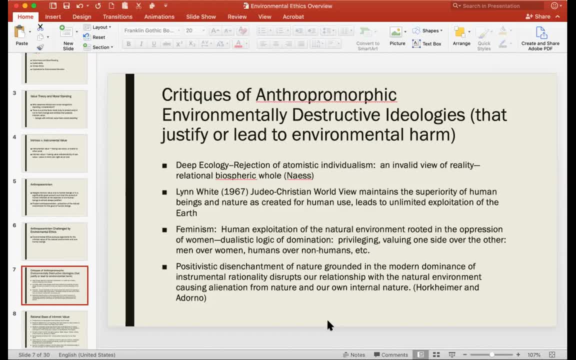 articulated originally by the norwegian philosopher arnie ness, and deep ecology, rejects atomistic individualism as an invalid view of reality and it favors a relational, biospheric, whole approach to uh, to reality that ness argued that we live. human beings live within a, as well as all other beings live within a relational uh hole that constitutes the biosphere. 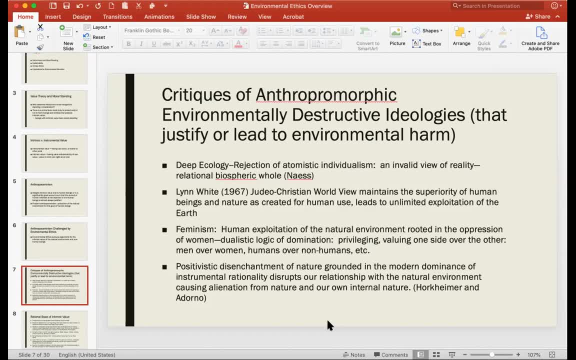 and therefore to take a human perspective. you, a human-centered perspective, is to uh, to violate reality and to cause harm lynn white, in one of the foundational pieces that launched environmental ethics in 1967, argued that the judeo-christian worldview, which maintains the superiority of human beings, 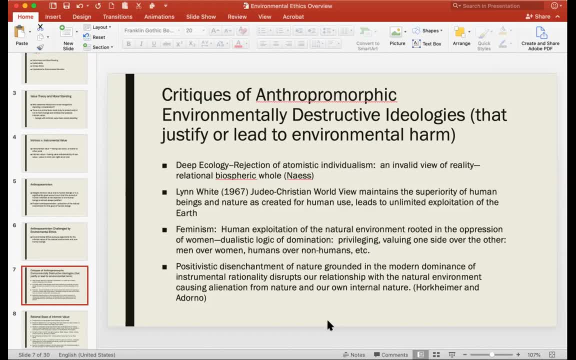 was highly destructive that the view that nature was created for human, human use. uh, in that, that worldview, that judeo-christian worldview, leads to the unlimited exploitation of the earth, white argued. a third critique is feminism, the, and a feminist critique of anthropocentrism suggest. 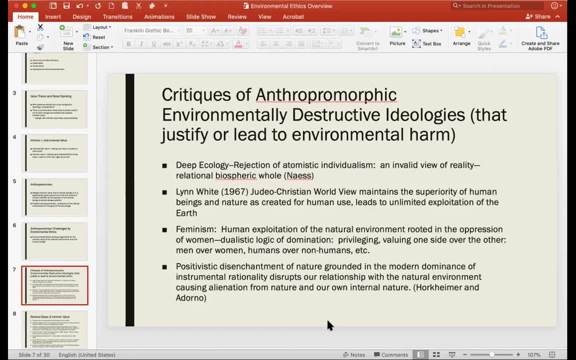 an interconnection between the exploitation of the natural environment and the oppression of women. that the exploitation of the natural environment was ran in parallel to, or was interconnected with, the exploitation of women historically. that there was a dualistic logic of domination inherent in patriarchy that exploited both. 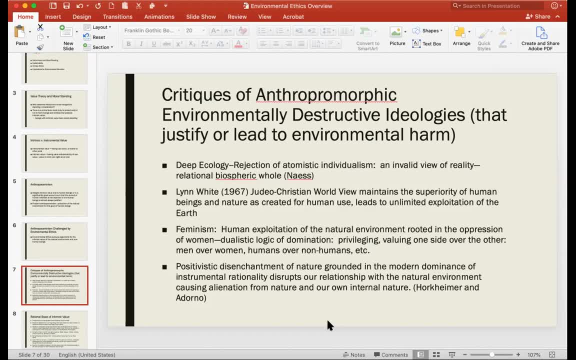 nature and female humans, giving privilege and value of one over the other, men over women, humans over non-humans, etc. So the dualistic, hierarchical thinking inherent in patriarchy was critiqued by eco-feminism to draw the connection between the exploitation of nature and the exploitation of women. 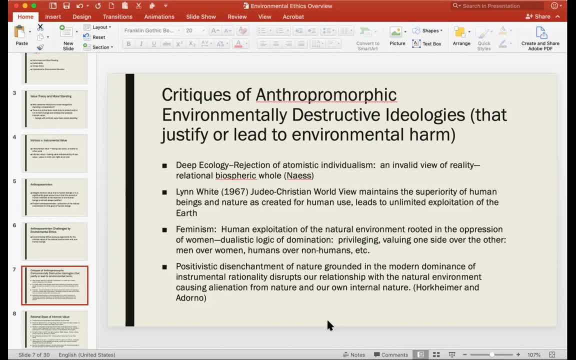 A fourth question, Critique came out of the Frankfurt School and critical theory that the disenchantment of nature, which emerged from the dominance of an instrumental rationality that characterizes modern thought and modern society, disrupted the relationship between the natural world and human beings and our own nature. 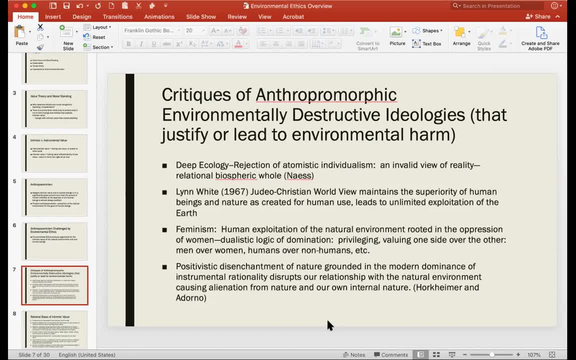 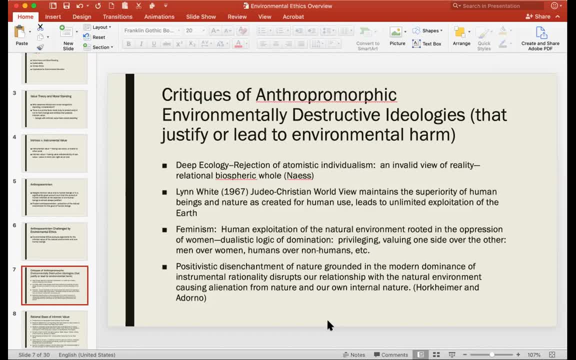 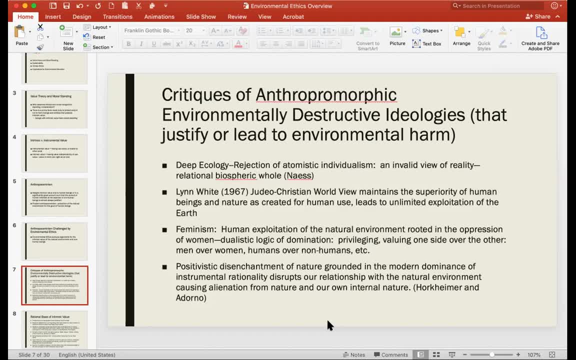 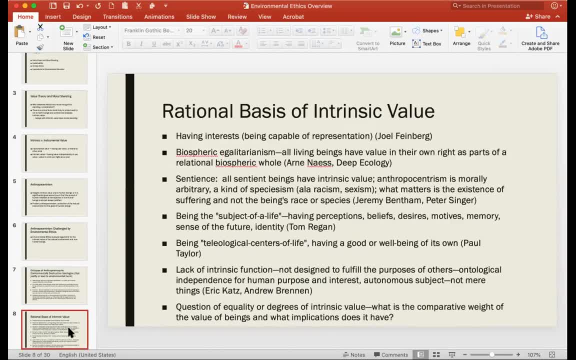 environmental ethics. There have been turning back to the idea of intrinsic value in moral theory. we would ask for the rational basis of intrinsic value. What gives us reason to hold others as having intrinsic value? And there are a number of theories, two of which will look. 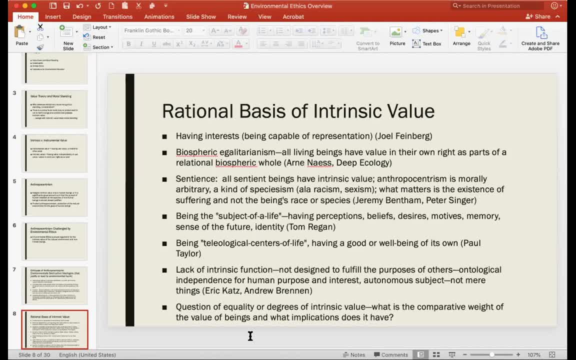 at in some depth when we meet again The singers, Peter Singer's argument from Sентиist as well as Paul Taylor's argument for beings being teleological centers of life. but there are a number of arguments for intrinsic value of nature and human and non human beings. 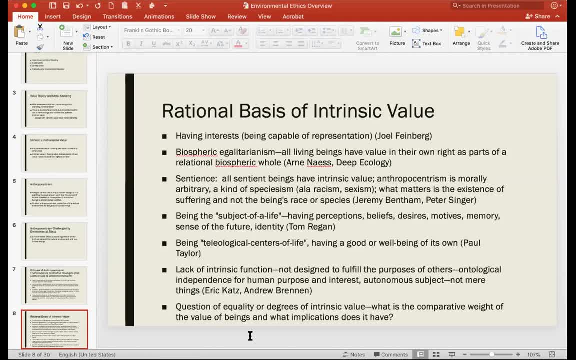 One is that They have interests and therefore are capable of representation. Having interests indicates that they have intrinsic value. Arne Ness says deep ecology is biospheric. Egalitarianism argues that all living beings have value in their own right as parts of the biospheric whole. 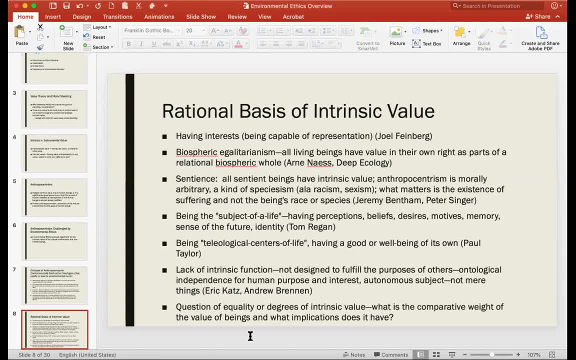 So all parts of the whole biosphere have value in themselves because they are part of this whole. An argument from sentience that all sentient beings have intrinsic value, That anthropocentrism is morally arbitrary because it's a kind of speciesism parallel to racism and sexism. 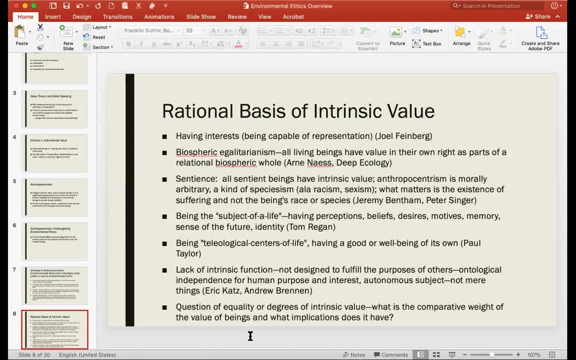 And that what matters is the existence of suffering and not the being's race or species. A fourth conception was being the subject of a life that is, having perceptions, beliefs, desires, motives, memory, the sense of the future, identity. That's kind of an offshoot of sentience. 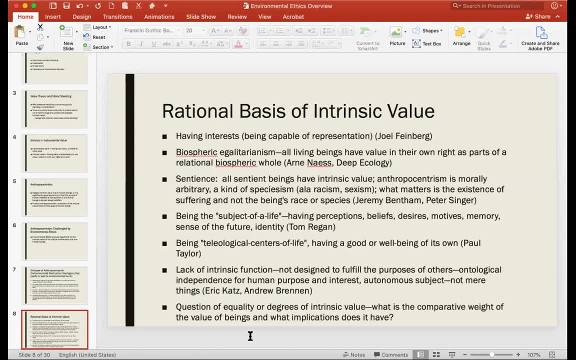 Paul Taylor's argument that beings who are teleological centers of life have a good or well-being of their own and should be considered to have possessed intrinsic value because they are alive and they are a center of life, That of life. Sixth argument for intrinsic value is that there is beings with an ontological independence from human purpose. 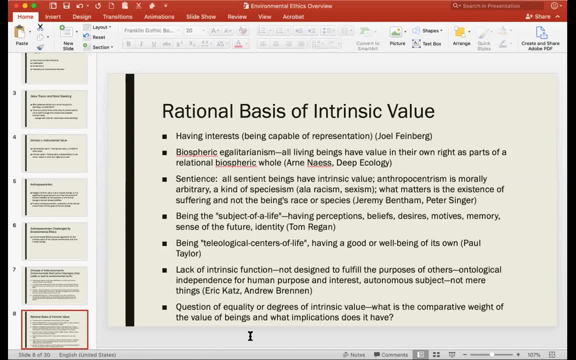 and interests are autonomous. They have their own life and interests and self-preservation. And they're not mere things. They lack an intrinsic function, That is, they're not designed to fulfill the purposes of others, They're designed to fulfill their own purpose. 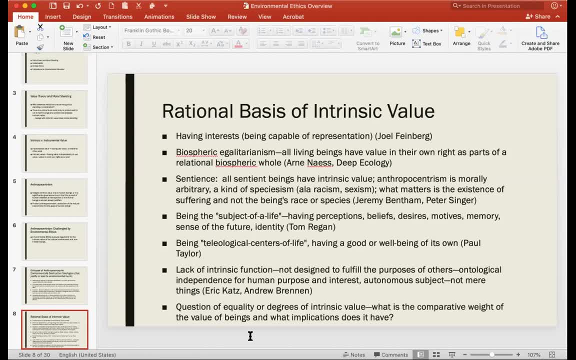 And finally, the question of equality or degrees of intrinsic value. We need to ask: what is the comparative weight of the value of beings and what implications does it have? If all beings have intrinsic value, are they weighted in any way? Is there any still any kind of hierarchy of value between them? 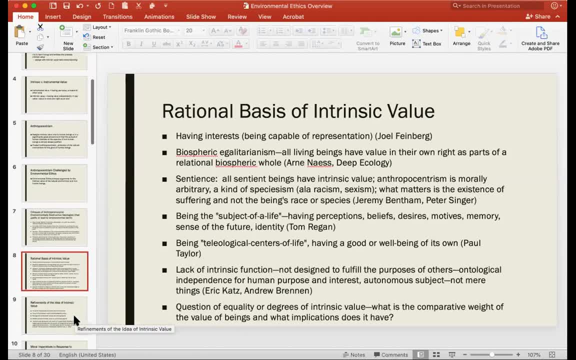 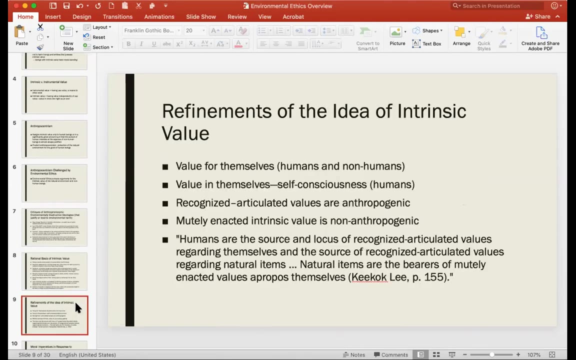 Is an elephant. does an elephant have more intrinsic value, a higher degree of intrinsic value than a mosquito, for example? Many of us would say yes. there remains a hierarchy of value among beings, Although Beings may all have intrinsic value. 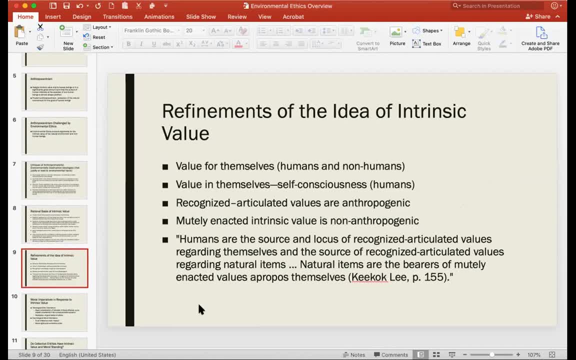 There's a certain refinement to the idea of intrinsic value and the distinction also between humans and non-humans, That both humans and non-human beings have value for themselves As they have an interest in the pursuit of their own value. But it's only. 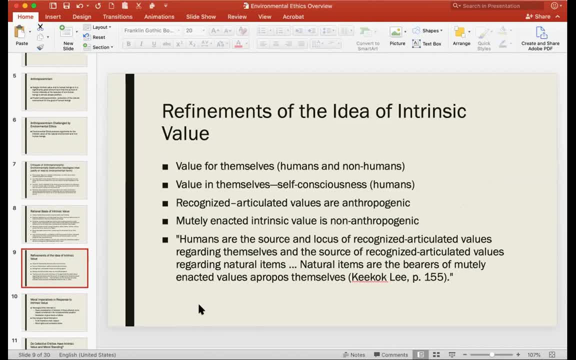 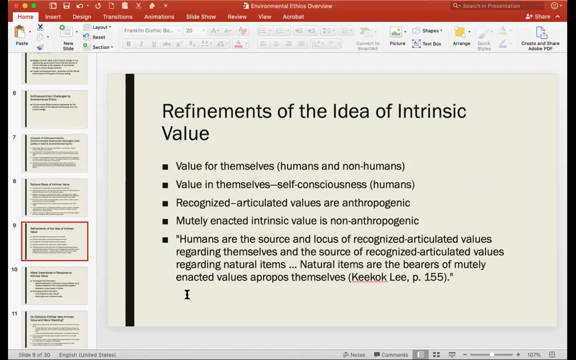 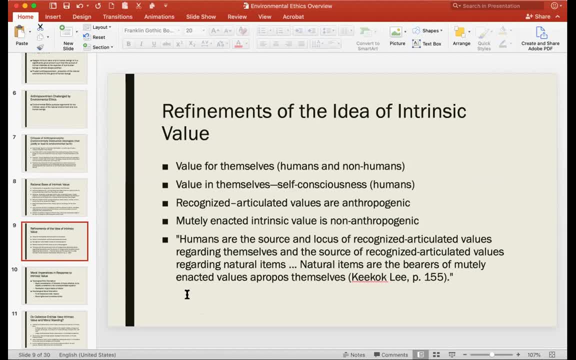 Is not anthropogenic, That is, it's not human created. So that's another distinction. It is argued that human beings Are able to recognize and articulate intrinsic value in themselves and in others, Whereas other non-living beings, non-human beings- 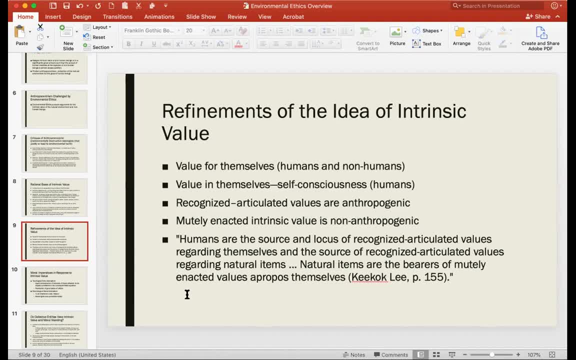 Are their intrinsic value is mute, It's mutely enacted, It's not articulated because they don't have the capacity to articulate the value. So Kikok Lee writes: humans are the source and locus of recognized articulated values regarding themselves and the source of recognized articulated values regarding natural items. 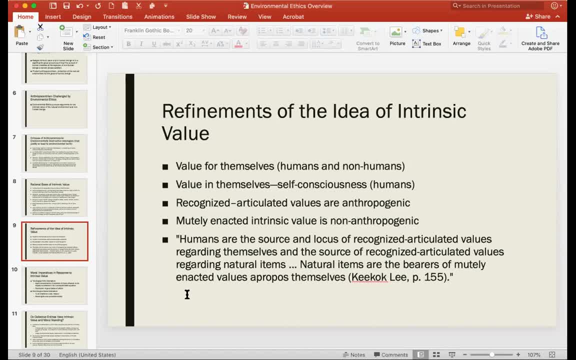 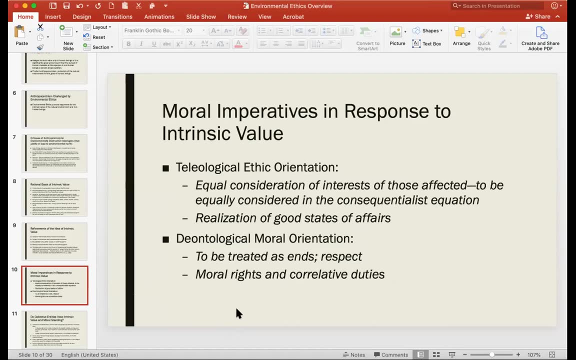 Natural items are the bearers of mutely enacted values. So And not recognized, articulated values, Following intrinsic value and the moral, ethical conviction of intrinsic value We can based upon our, The moral point of view, We would derive Consistent. 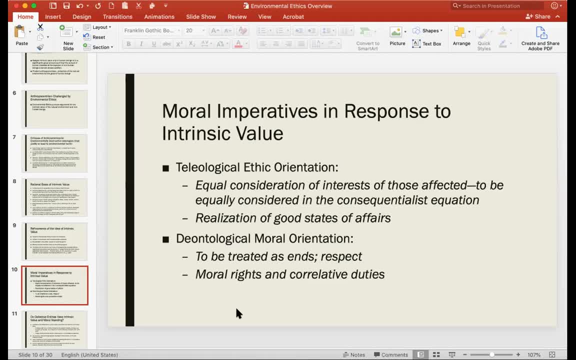 and coherent moral imperatives would be derived from intrinsic value. and there are two basic orientations to moral principle. one is the teleological orientation, which defines the good and then defines what is right in terms of real, the realization of that good, and this is often expressed in terms of the equal consideration of interests. 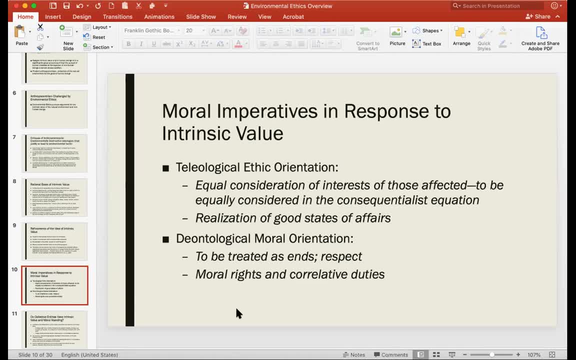 of those affected to be equally considered in in the consequentialist equation. so the teleological orientation is consequentialist and it looks to to define the right in terms of the realization of the good as states of affairs. an alternative moral orientation is the deontological orientation, which defines the right independently. 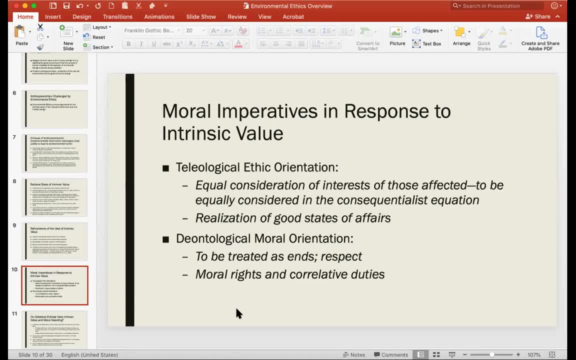 of the good and defines the right in terms of relationships between beings, human beings and other beings, rather than the realization of some good state of affairs and the. the deontological orientation suggests that those with intrinsic value uh are to be treated as ends and to be respected as ends, and from that that uh respect for persons or respect for. 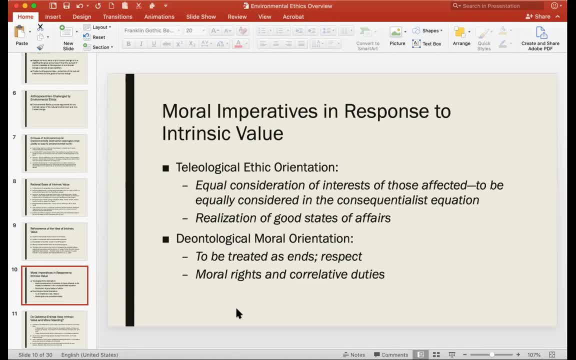 living beings is derived to moral rights and uh and duties, correlative duties. so there are, and both of these orientations are, have a lot long histories and they're uh both, uh, they're both reasonable positions uh to take, but distinct in in certain ways. one, the teleological, seeks to actualize or realize the good. 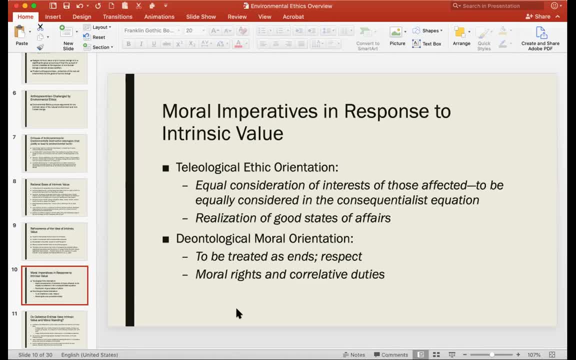 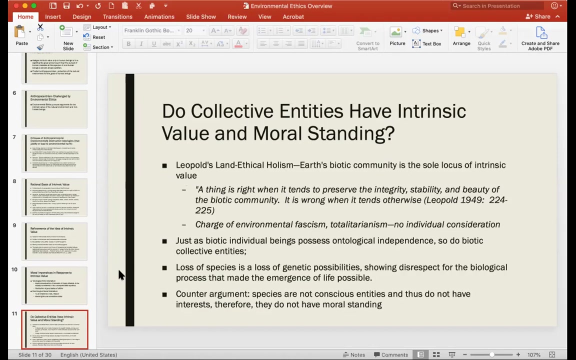 the deontological approach looks to relationships rather than realization and and respect for beings, human beings, and the deontological orientation is to define the right, in terms of relationships at that, from which uh moral rights and duties are are are derived. Dr Starwood, can you? can you repeat that last part just one more time, please? you uh froze. 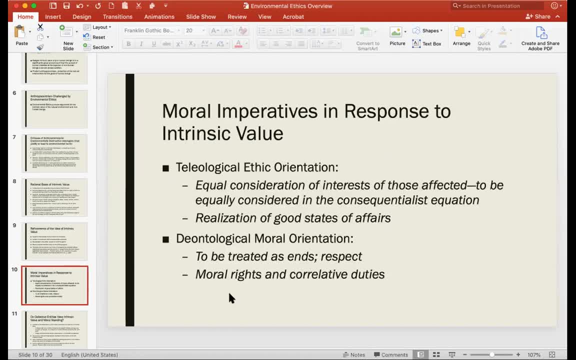 oh, okay, uh, the deontological- yes, yeah, and a deontological orientation looks to how uh to relate to the good and the bad relationships rather than the realization of states of affairs, and uh seeks to have uh respectful relationships as the foundation of uh of morality, as opposed to the equally considering interest in. 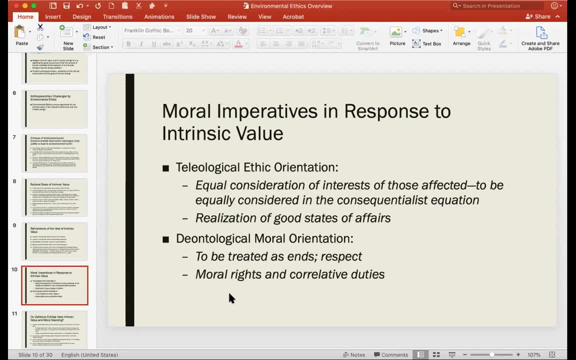 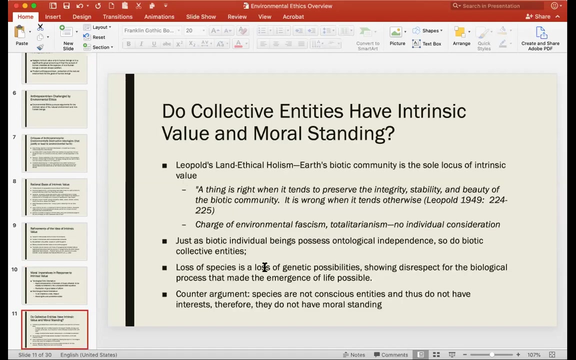 some kind of calculation about the uh, some kind of calculation about the realization of some basic good. so those are uh, two orientations that are are different ways of thinking about what is what is right. does that make sense? yes, thank you. okay, uh, that leads us to the question of uh. do collective entities have intrinsic value? 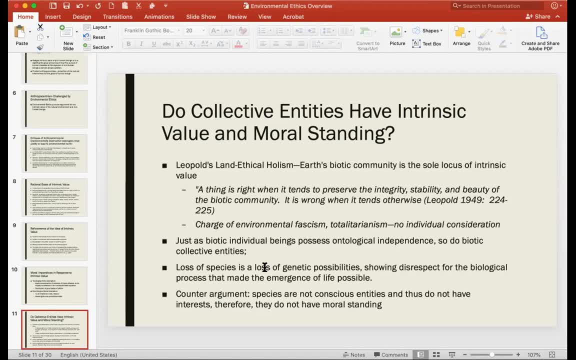 or is our only individuals? individual beings are the ones that are intrinsic to the value of the biotic community, the biolog globe. and then we can come back to this as a full-scale question, and i shall pass the question 자문 forth. is that, uh, working? you know again, thanks to, uh, Dr Starwood. um, now then, be careful with what i am speaking from. 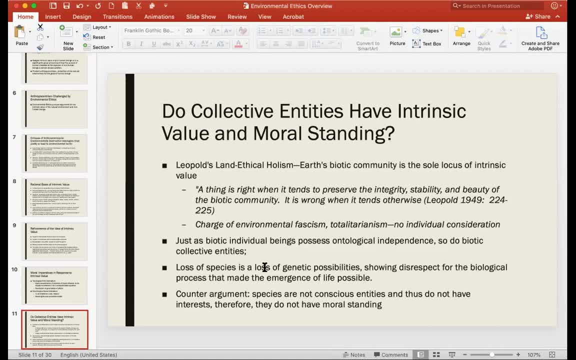 the whole natural environment to be having intrinsic value. And his famous principle was: a thing is right when it tends to preserve the integrity, stability and beauty of the biotic community. It is wrong when it tends otherwise. Some have argued this is a kind. 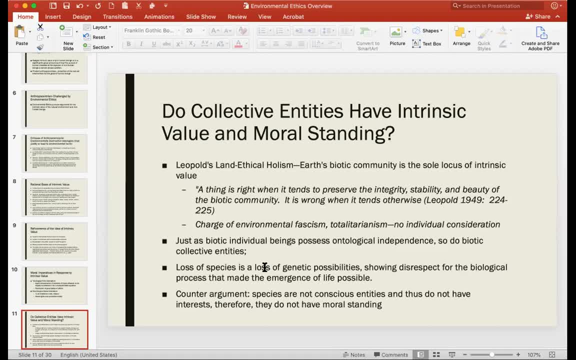 of environmental totalitarianism that doesn't give any consideration to individuals. But the argument is that just as biotic individuals possess ontological independence, so do biotic collective entities. There's a argument for the moral standing of species based upon the loss of genetic possibility. 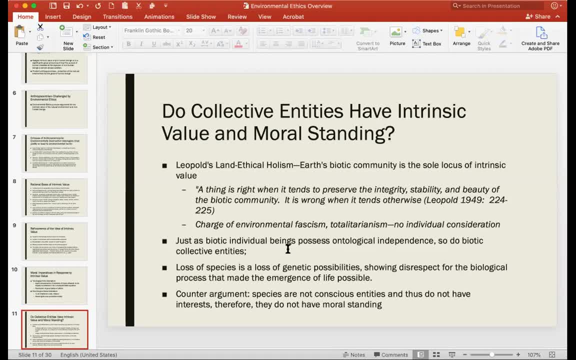 that when a species becomes extinct, that their genetic possibilities are extinguished, and that shows disrespect for the evolutionary process that makes life possible. The counter argument- and this is offered by Springer, for example- is that species are not conscious entities and thus do not have interest. 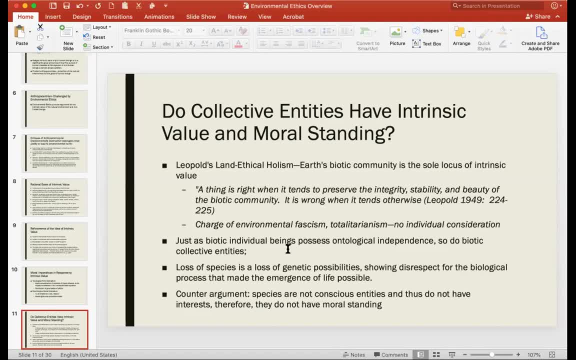 And therefore they do not have moral standing. Only beings that are sentient can have moral standing, according to Singer, And species as a whole are not conscious as such. So that's a big question: The value of nature and the value of species. 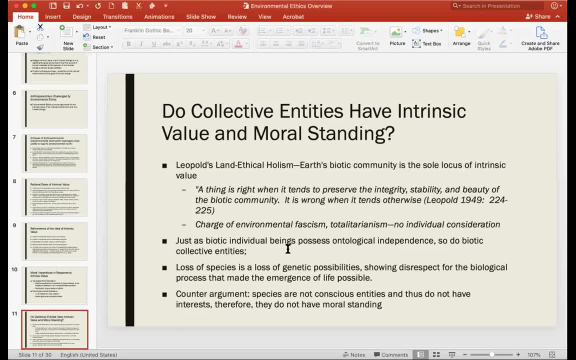 of landscapes, of biotic communities, of the biosphere itself. Do all those have intrinsic value? And we'll look further into arguments for the intrinsic value of species and biotic communities and natural landscapes, et cetera. Dr Snodward, may I ask a question please? 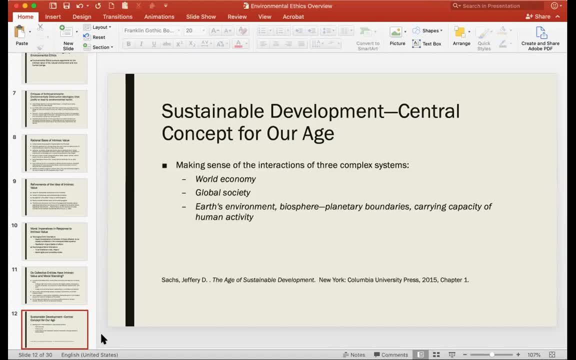 Sure Can something have both intrinsic value and development value or instrumental value at the same time, Yes, yes. So human beings, for example, have both intrinsic value. We recognize their intrinsic value, but they also have instrumental value. I have instrumental value to you. 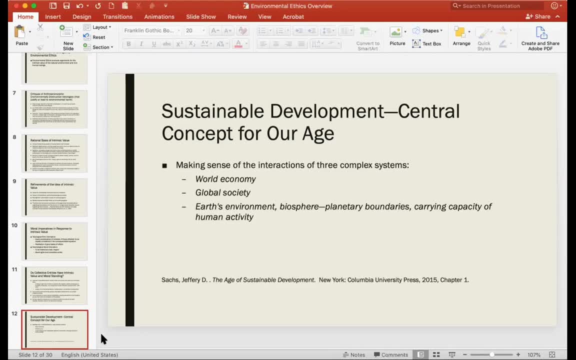 To me? yeah right, In the sense that I can offer you knowledge, understanding, et cetera, Or you have intrinsic value, Instrumental value, to others when you're employed by others. So one more question: To do some work. 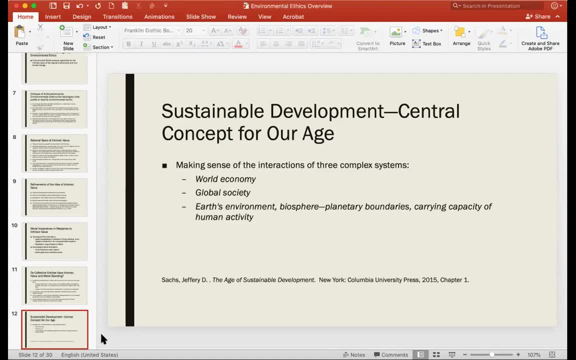 Oh sorry, One more question. So what about who decides something has intrinsic value, Like instrumental value? it's easy to understand, but how do you decide that this thing, the entity, has the intrinsic value? Who decides that? Well, human beings pretty much decide that. 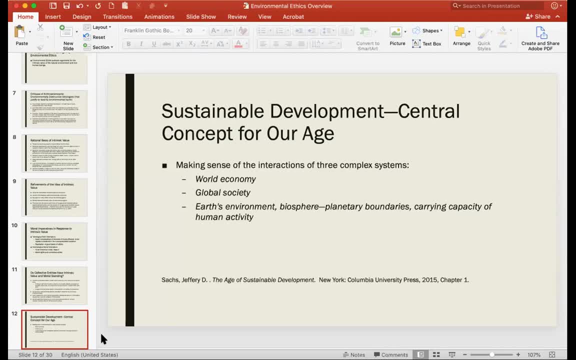 Oh, okay, And that's a part of ethical and moral reflection into our relationship with ourselves and with other living things. Okay, Are there reasons, are there grounds that would justify our perceiving other beings, non-human beings, as having intrinsic value? 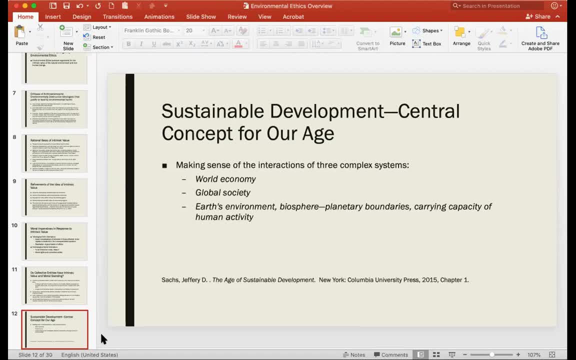 And we listed. we discussed a number of them earlier. Sentience is one argument. Another argument is that a being that is a teleological center of life is also to be considered as having intrinsic value and moral standing, et cetera. Thank you. 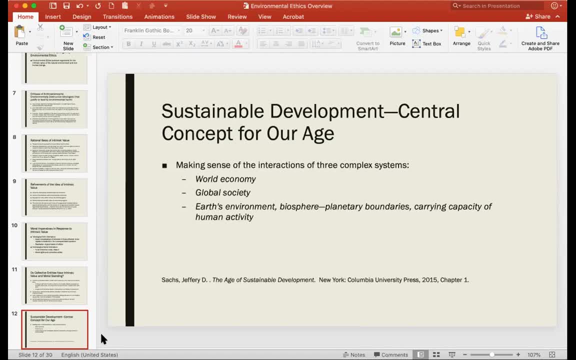 I had a question: What about humans that have like, maybe like developmental, like delays, or like they're not aware of some, so like, how would they fall into these, this type of thinking, you know, cause maybe someone is just born with a delay of some kind? 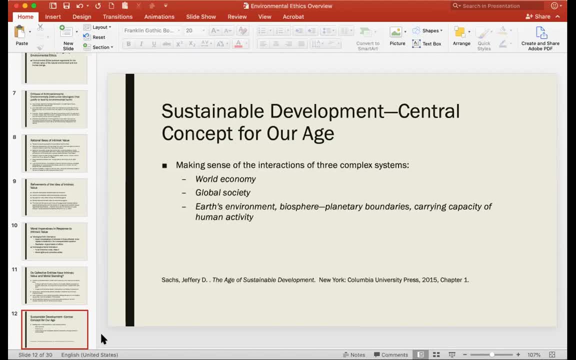 They're not aware of every single thing. I don't know if that makes sense, though, but I was just thinking about how would that fit in? Well, we would argue that, for example, from sentience, that all human beings who are 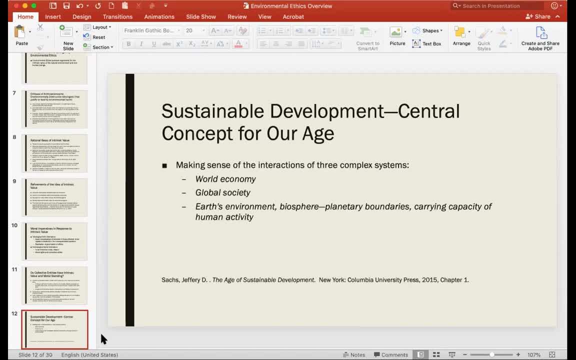 well from sentience is the person capable of experiencing pleasure or pain, even very rudimentary, And we would most conscious human beings, or all conscious human beings, have the capacity for suffering or for enjoyment, even if they are limited in their genetic. 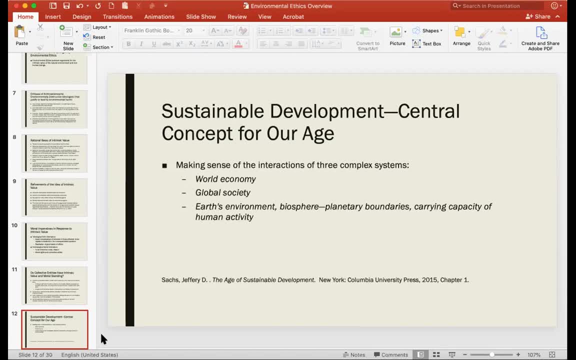 or biological capacity due to some damage to their genetic makeup. Dr Sauer, could it also be argued, aside from intrinsic value, obviously instrumental value, with the viewpoint of these people, providing opportunity for growth for their loved ones or for you know, for the parents of the children? 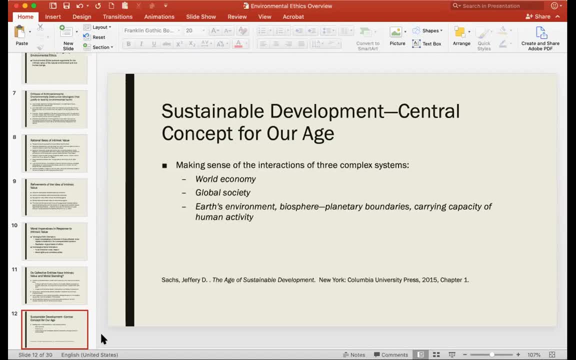 I know that's very philosophical, but I mean, couldn't that be argued as an instrumental value as well, how people with certain disabilities being in our lives provide opportunities for growth for us as well? Yes, I think so. Yes, They would have an instrumental value for us in that sense. 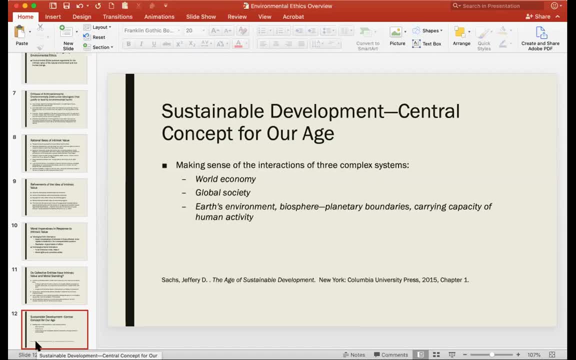 But we would also recognize their intrinsic value Absolutely, Either as sentient beings or as really living beings, Like, for example, people, human beings in comas, for example, who are not conscious in that moment. We still have an obligation, you know, to be conscious. 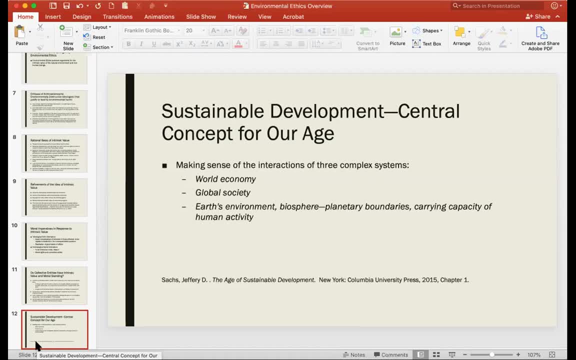 Many would argue to treat them with moral respect and not unless they have pre-established a living will, for example, to not be kept alive mechanically. we would keep them alive as long as possible because they're living, And that's a recognition. 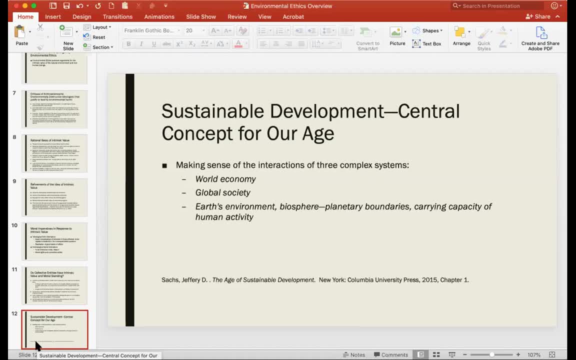 of their intrinsic value, in their moral standing. so if it's a very like a severely handicapped person, like we don't know if he knows the pain or not, but he or she can teach us the love, so we would consider that person has the instrumental value because he or she teaches us patience and love and you. 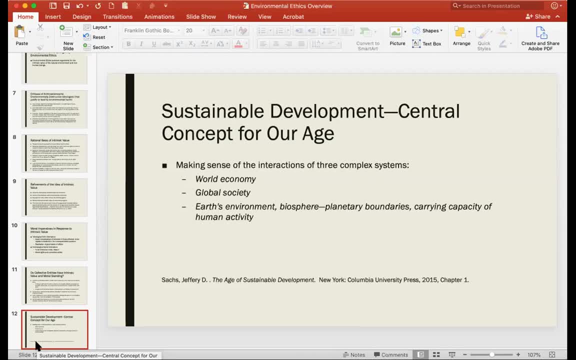 know right, that's instrumental, because there are. there are means, they're providing some kind of means to our, our ends and- and that's calm, that's of course common in in our interaction with each other, we're often providing instrumental value to each other. can, can the concept instrumental value be mutual as a mission between two? 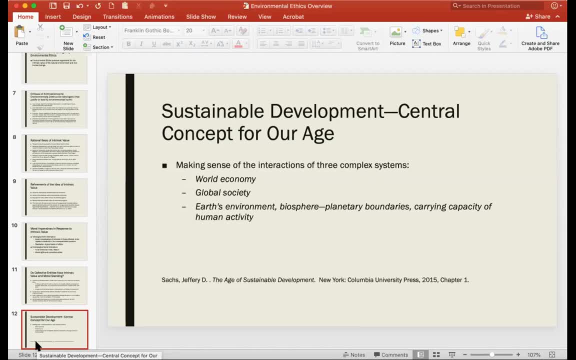 aspects, for example, between professor and the student, between me as a human being and trees, for example, can each, each one of us on his side, has instrumental value to the other? yes, yes, we are, and that's very common and we are. economic relationship, for example, is based upon mutual instrumental value to each other. I will 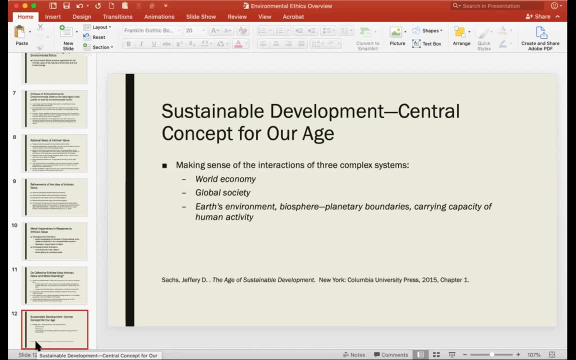 I will provide you X service if you pay me X amount of money. my car breaks down. I take it to the shop and I pay. I make an exchange right for the service, the services to fix my car, in exchange for the property that I have. 그런데 I make in exchange right for the services to fix my car in exchange r. 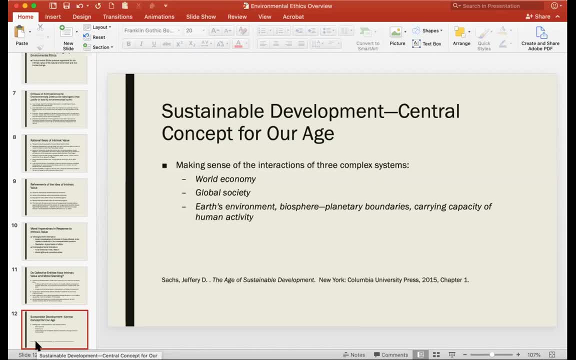 car in exchange right for the services to fix my car in exchange r for the services to fix my car in exchange r for for a certain payment. so were you, in that case where we're both using each other instrumentally, but we should- you are the mutual instrumental value that? 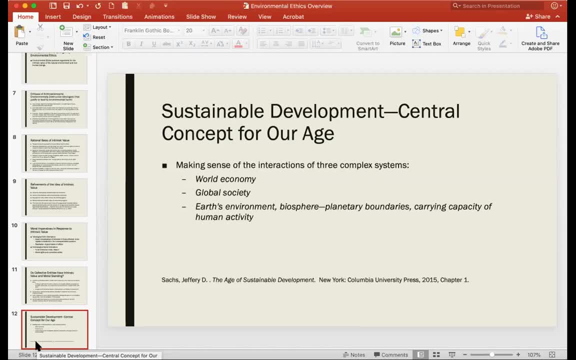 we exchange should remember more from the moral point of view, should be based on respect for our intrinsic value. okay so, and that would prevent us from being unfair, unfairly exploiting someone, or the mechanic cheating me or I cheating them. that would violate their status as intrinsic, having an intrinsic value in 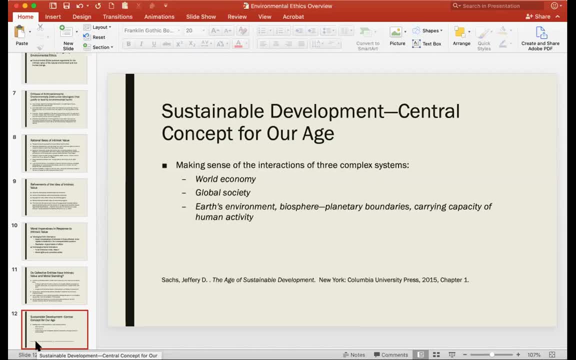 our instrumental relationship. so the instrumental value is is a moral conviction that is perhaps foundational to our ethical and moral relationships with each other and and potentially, with other other living things. so do we? do we take into consideration other living beings when we make our choices to cut down a forest, to 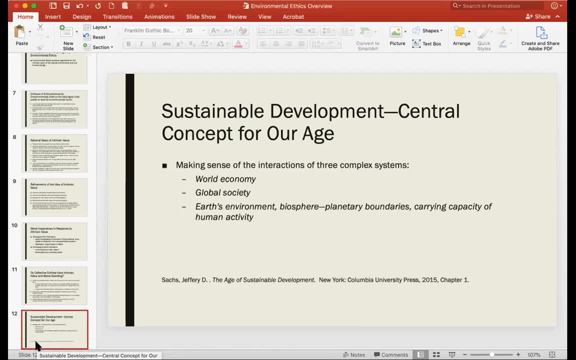 pave the way for a parking lot or a new shopping mall? should we take into consideration they, the other other living things there, from an environmental point of view and an environmental ethical point of view? the argument is that we should take into other living the the well-being of other. 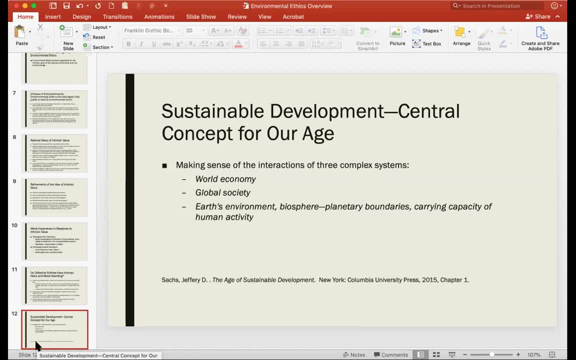 things, other living things, into consideration, as we would take into consideration the well-being of others and the responsibility that we have for welfare and theייne for us to be able to be accountable or open to the being of other human beings when we act in the world. so that's- uh, that's a basic, that's the basic. 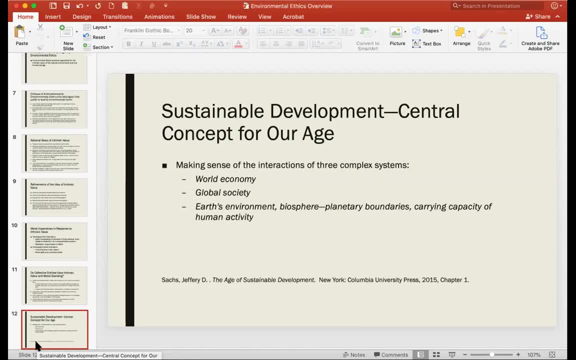 moral point of view. does that make sense? yes, thank you. so our um intrinsic values are, though can those also be values? could that also be something that we value? yes, okay, so like as far as then say, for example, if, uh, we value family, value, honesty, value love. 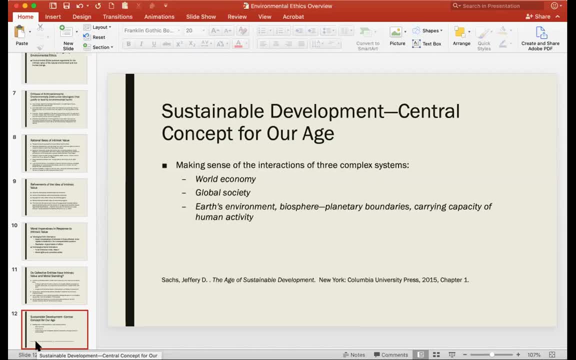 yes, okay, yes, so it's a. it's a. it's a recognition of the value of others, okay, who have those uh, who potentially have also have those desires. you know who have those uh, who potentially have also have those desires and and uh expectations. all right, it's, it's um. that moral conviction is uh is an answer to the question: why be? 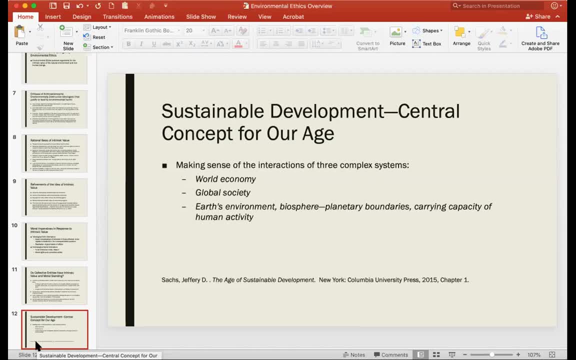 moral. why should i consider, why should we consider, the well-being of others? one answer is that they are beings like ourselves who have value in themselves and shouldn't be uh and should be morally considered, should be morally respected in relating to them. sorry, our, our, our, recent uh, uh, recent events of police brutality in in the United States of of. 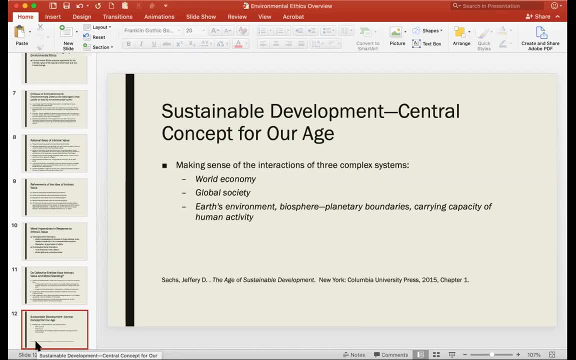 killing, uh, without due cause, without justification. that's wrong- innocent african-american men and women by the police. it's a profound. it's a profound violation of their intrinsic value and their moral standing, and as well as we, and, and so that's why it's so outrageous. right, it's where it's, it's so. 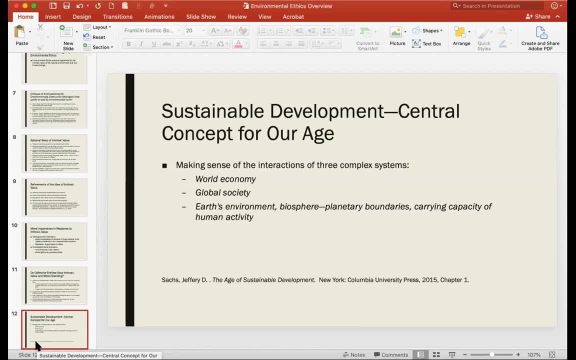 basically disrespectful. basically such a basic violation to take another person's life without cause or is, uh is the worst kind of violence and the worst kind of of moral injustice. and so we're right to be african-american people, are right to be totally outraged by this. 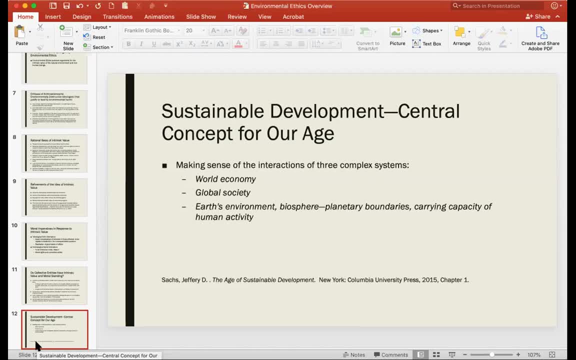 as well as everyone else. so that's an example of you of the importance of seeing others as having seeing others as ends rather than as means to to our ends. to see them as, but possessing intrinsic value rather than only instrumental value makes sense. i have something that i know americans always try to avoid to 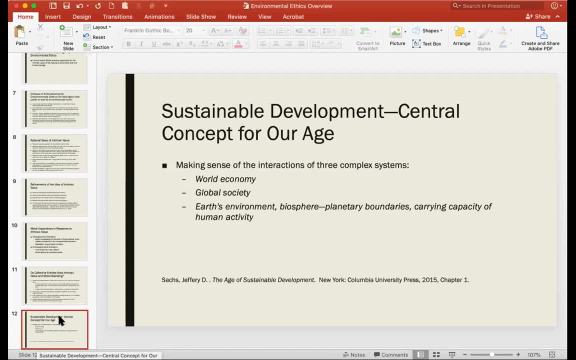 talk about. but you know, being me, i i'm sort of challenged my view now. so let's say the abortion view. so basically, this is really pro-life if you're thinking about someone's instrumental value. so who has the right to terminate, no matter how early stage, it is right. wouldn't that be a? 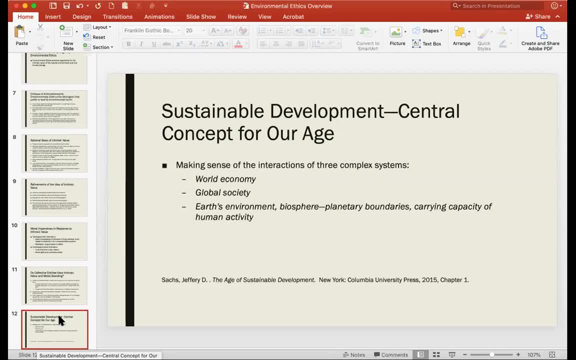 violation of ethics. well, it could be, that could be argued right, but is there is a um, um, that's a? i know people don't like to talk about it. you know when? when does human life begin? does human life begin at conception or at, uh, at a later stage of development of the fetus? okay, okay, that makes sense. 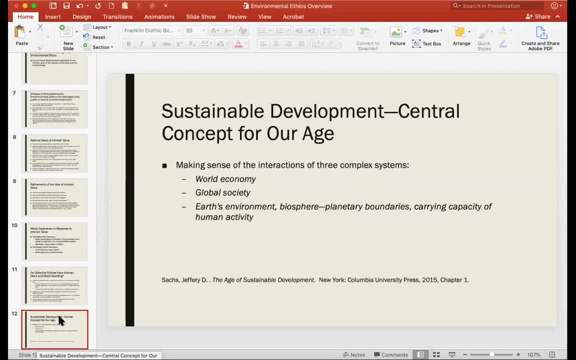 uh, when, when is there another being uh separate from the mother? uh, and does a mother have uh have also rights? right, uh, to be self-determining, to determine her own, to have control over her own body. so that- and it's a stick- very difficult moral dilemma. right, right, very and very uh heated. 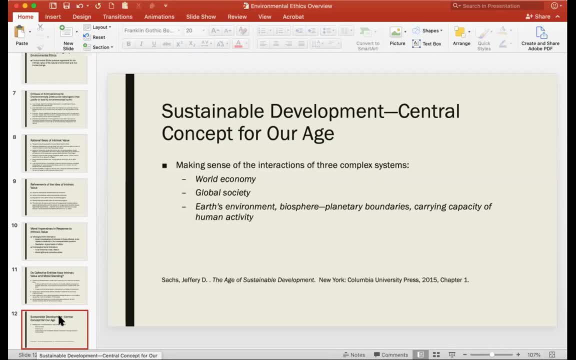 moral dilemma, but uh, and i think it, it hinges on, uh, certainly, the fetus at some point in her life, at some point, is a human being and has intrinsic value. um, but is a? um, you know, a undeveloped, is a fetus in the third week or fourth week. 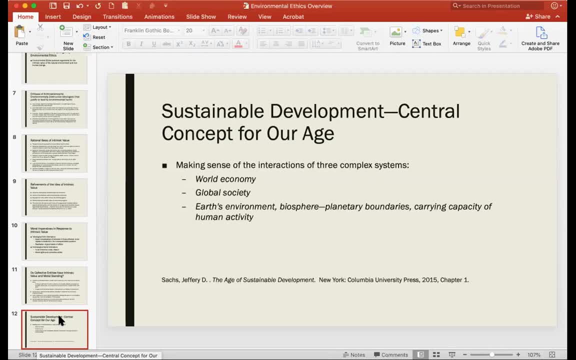 or eighth week, uh, a human being that's distinguishable from the mother's, from the mother? okay, is the question. okay, that makes sense, thank you. and and in the law, at least in the united states states, the law so far- has placed the right to choose as more fundamental. 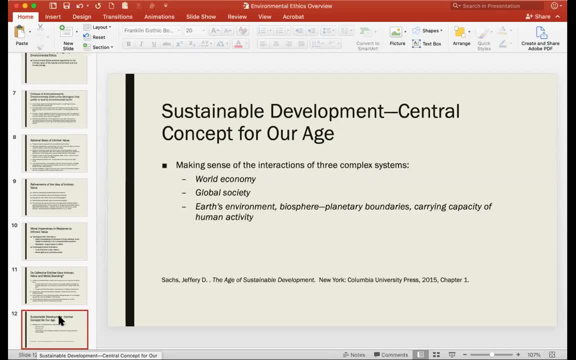 at a beyond a certain stage of development of the fetus or limited by a certain stage of the fetus. other societies have different points of view about about that, but it boils down to when: when life begins, when they're, and when human life begins. so that's- uh, that's a difficult one. 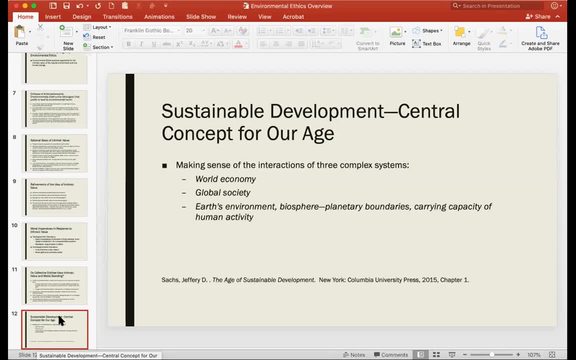 so uh, another dimension of environmental ethics, less foundational than the consideration of intrinsic value, is uh and moral principle that derive from intrinsic values, the idea of sustainable development and, in the consideration, the ethical and moral duty to uh have economic activity and social activity that is sustainable in terms of environmental capacity. 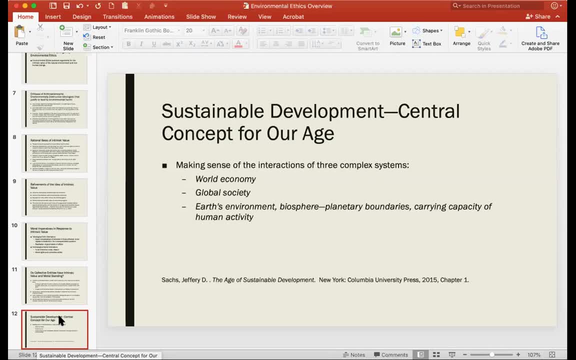 and uh. sustainable development involves complex systems of economy, society, in interaction with the Earth's environment, its biosphere, And sustainability refers to the carrying capacity of human activity And it's a question of what are the limits to human activity If we go over the limit of the carrying capacity of the environment? 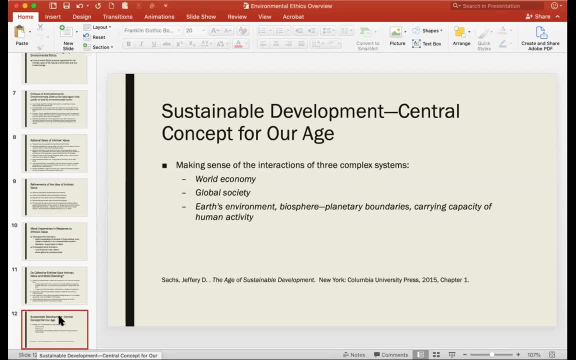 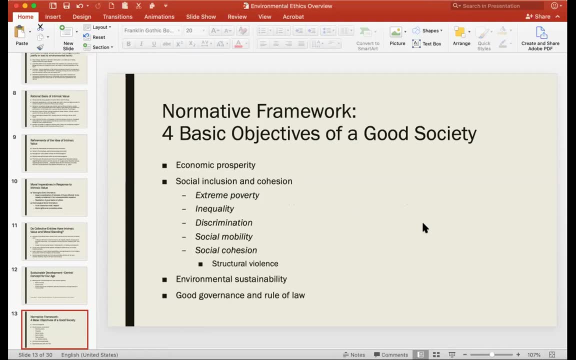 then our activity is not sustainable. That's a very important consideration And it involves, it's a part of a particular normative conception of a good society. That a good society would include would guarantee economic prosperity, would guarantee social inclusion and social justice. 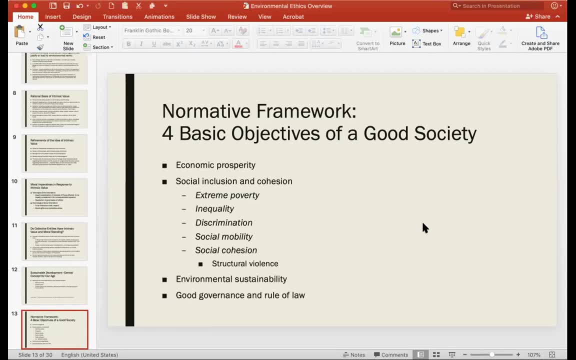 would guarantee good governance and the rule of law. and fourth, and this is relatively new, a good society, a just society, would also be environmentally sustainable over generations. And this, the idea of sustainability, links to issues of environmental justice about the burdens. 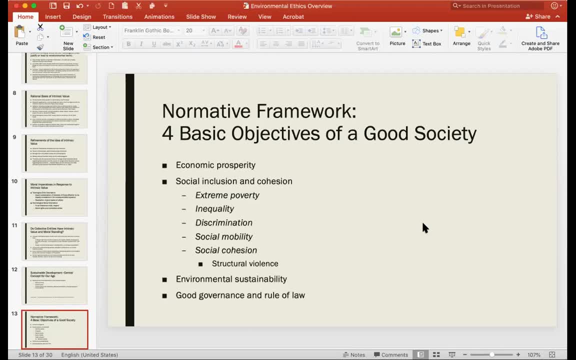 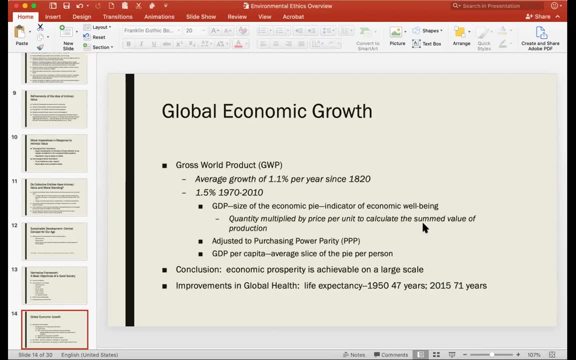 who benefits and who is burdened by environmental sustainability and environmental destruction. So, if we look at the question of sustainability, economic growth is of critical importance, And that we have. it has been demonstrated historically that economic prosperity is achievable on a large scale. 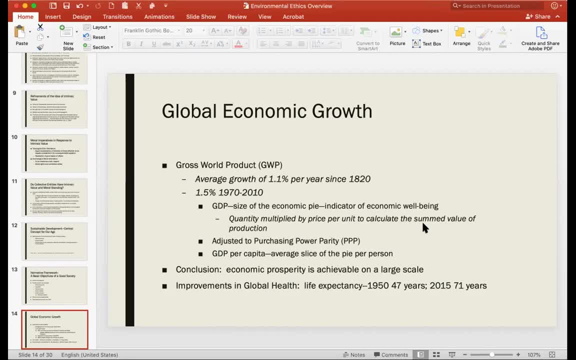 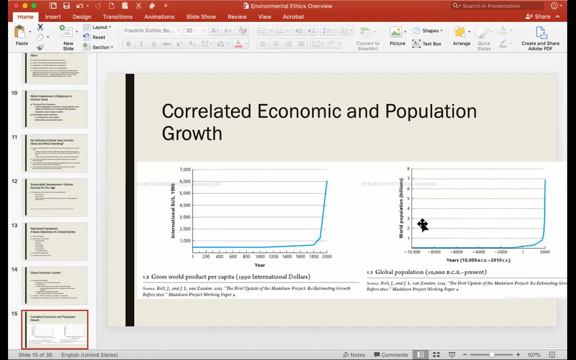 There's been an average growth in the United States of America in the last few decades. There's been an average growth of economic prosperity since 1820. And the size of the economic pie has expanded since the beginning of the industrial revolution. So we can see global economic growth and population growth are correlated. 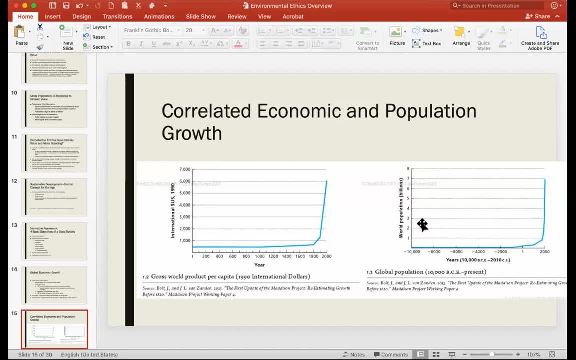 And really we've had an enormous increase in economic growth, In industrial, in economic activity since the beginning of the 19th century. Economic productivity was very low and very stable over centuries. From the year one to the year 1800, there wasn't much change in the productivity of human beings. 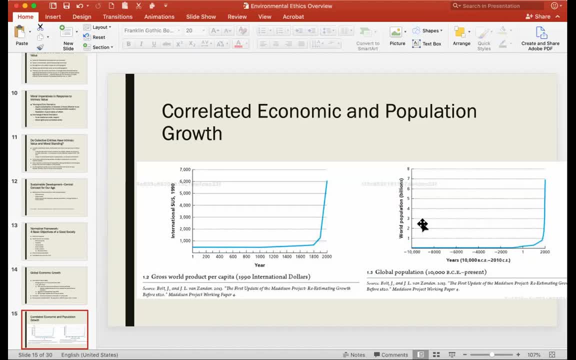 But that took off exponentially at the advent of industrialization. the application of science and technology to economic development And the growth in economic activity is parallel or correlated with population growth, which has also grown exponentially, beginning in the late 19th century and into the 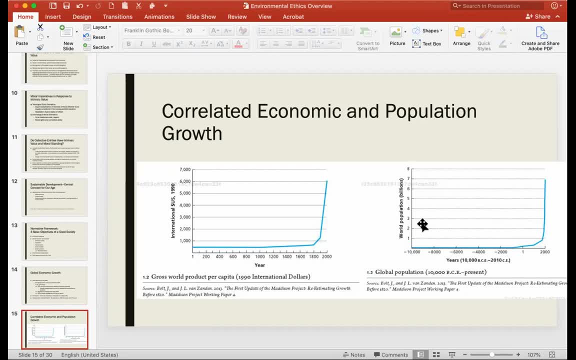 the 20th century and the 21st century. There was very little population growth in the past 10,000 years up until the advent of the industrial revolution, And that has grown exponentially. So we've entered a period, in the last 200 years, of great economic activity and corresponding growth. 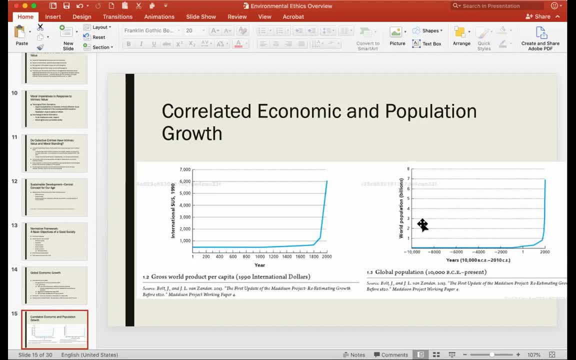 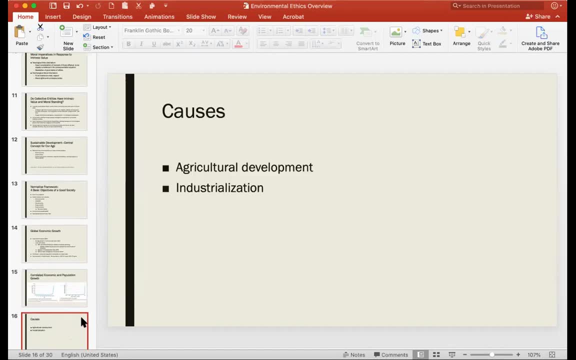 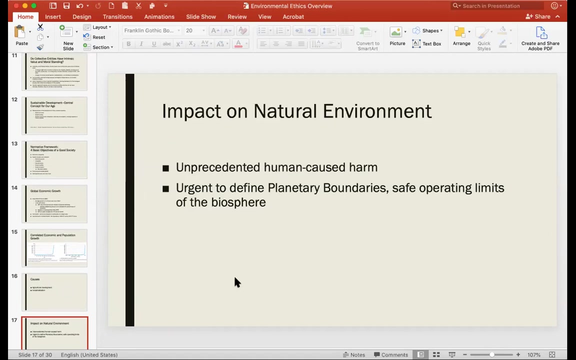 in human population And that has been basically caused by agricultural development, the production of surplus food, as well as industrialization, And this growth of economic activity and the growth of human population has had an enormous, enormous impact on the natural environment. There's been unprecedented human cost harm to the environment and resulting in the urgent demand to 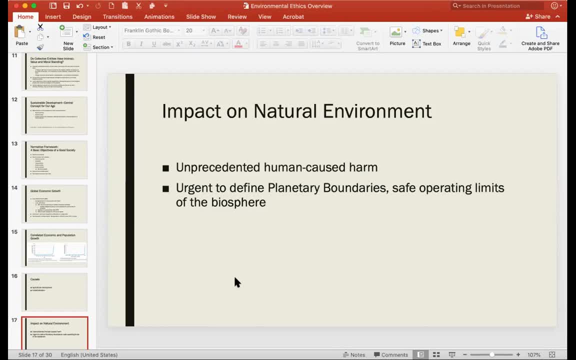 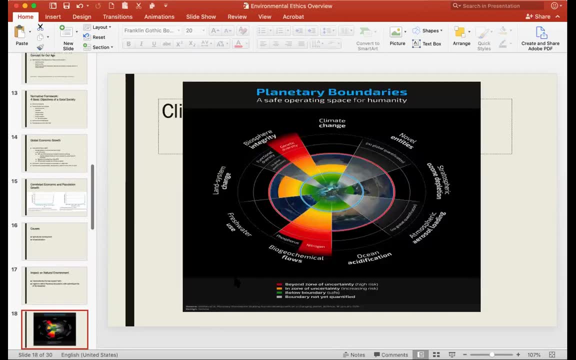 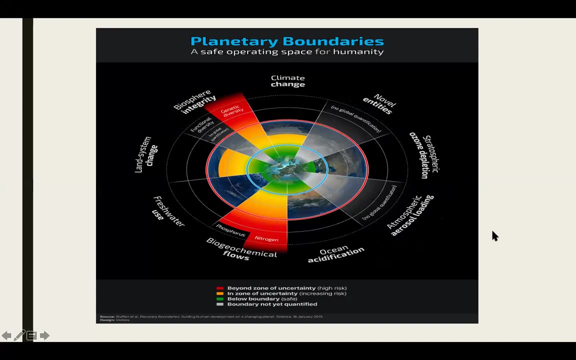 an urgent need to define what the boundaries of the planet are. what are the safe operating limits of the biosphere? And this is? scientists have have attempted to begin to map the planetary boundaries and the limits of the carrying capacity of the biosphere to carry human activity and where we might be. 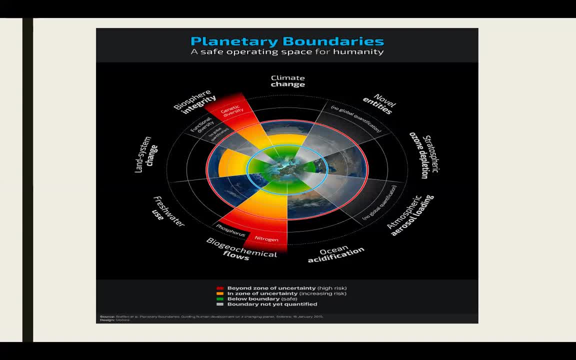 going beyond the boundaries of the planet. So there's a lot of work to be done. There's a lot of work to be done. There's a lot of work to be done That are safe For both human human beings and safe for other living things and the biosphere itself. 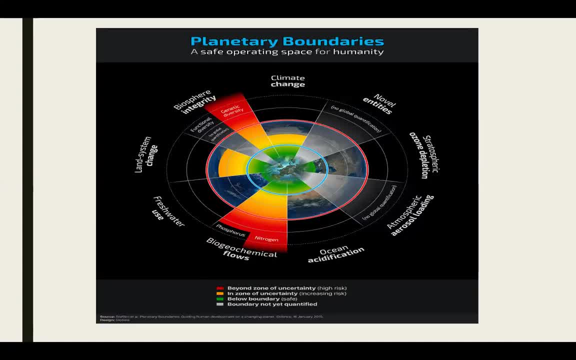 So sustainability is about Knowing what these boundaries are and limiting our capacity or our activity to stay within the boundaries of the biosphere, The carrying capacity of the biosphere- and we're in danger of danger of exceeding those limits as our activity increases. our economic activity increases. 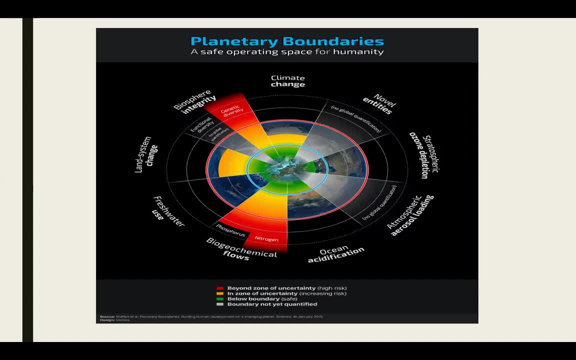 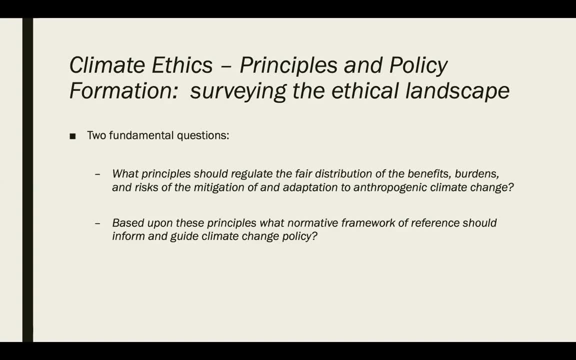 and our consumption increases and the human population expands. And one element, a very important dimension of sustainability and dimension of planetary boundaries, is the effect on the climate caused by carbon pollution in the environment, That is, the burning of fossil fuels- coal, oil, natural gas, et cetera- have increased. 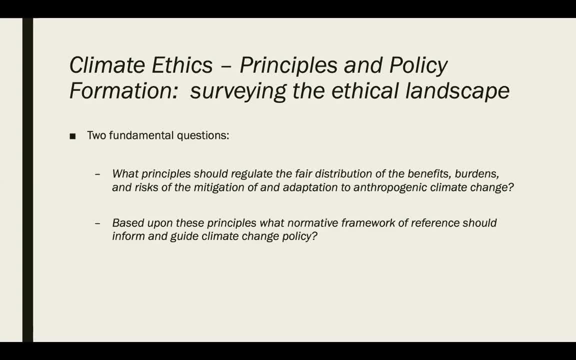 the amount of heat trapping material And the atmosphere, exacerbating the greenhouse effect to the point that the climate is changing. the planet is warming due to the greenhouse effect and the increased amount of heat trapping material in the atmosphere, And that includes an increase in water vapor. 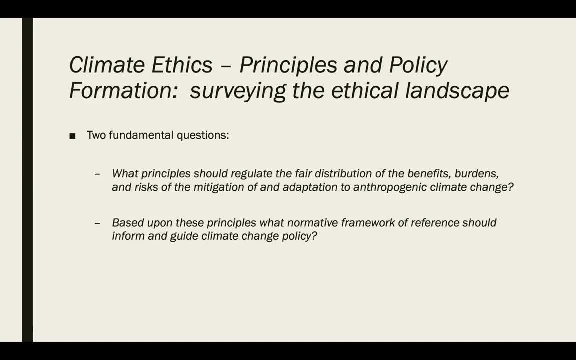 In the atmosphere, Which also traps heat. We'll talk more about climate change in the near future, But the fact that there is human-caused climate change, a human-caused global warming, gives rise to two fundamental moral questions or considerations, And they are: what principles should regulate the fair distribution of the benefits burdens? 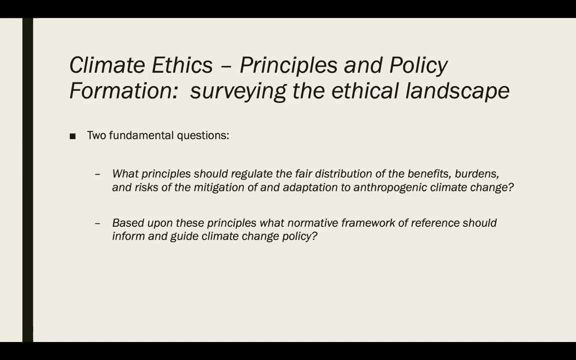 and risks of the mitigation of and adaptation to climate change And, based upon these principles, what normative framework should inform and guide climate change policy. So climate ethics has to do with principle and, as well as principles, that info inform any policy that, хотя taa naauce the aging climateiamiicek as a basic, рублей at the 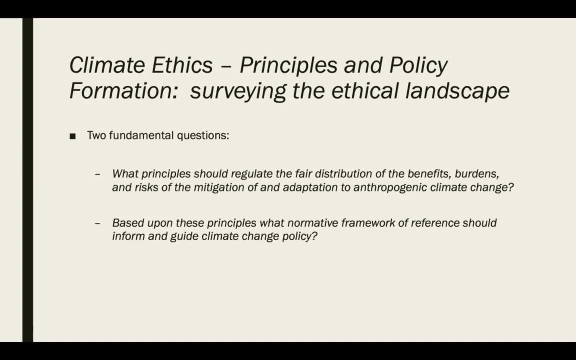 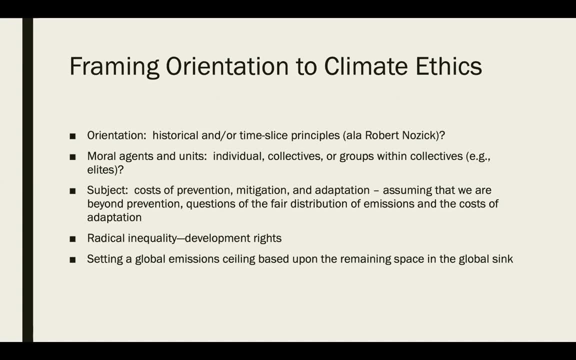 Aim Amongst �91. As well as principles that inform and guide policy and climate change, And we'll have a little project of risk mitigation: Cairo, Ms B Shannon, who is an electorate when you think of these things that inform our response to climate change, and there are a number of further. 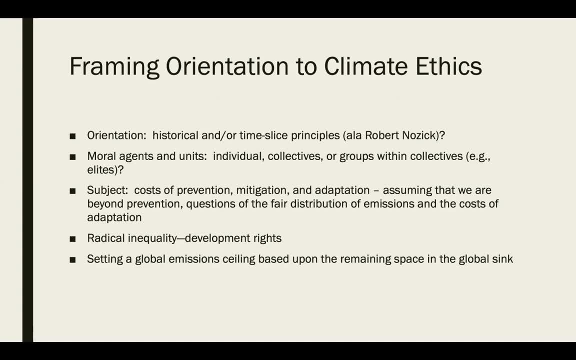 questions involve us, as we'll explore later, whether we our orientation, whether we look at the history of carbon pollution or that we take a point in time like 1950 as the starting point for considering the benefits and burdens of climate change, or do we go back to the, the beginnings of the Industrial 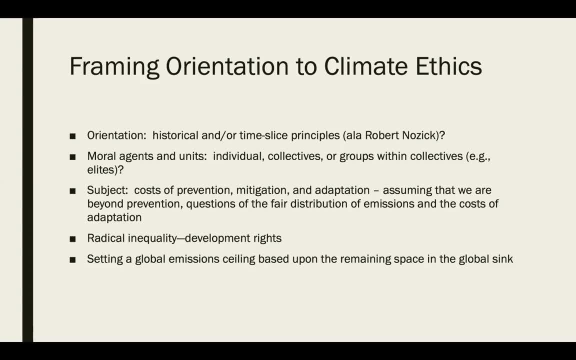 Revolution. a second consideration is whether moral agents and unit what? what moral agents and unit should we consider in thinking about climate and climate ethics- individuals and communities, and how do we think about climate and climate ethics- individuals, collectivities, groups within collectivities? we should also consider the costs of prevention, mitigation and adaptation questions of 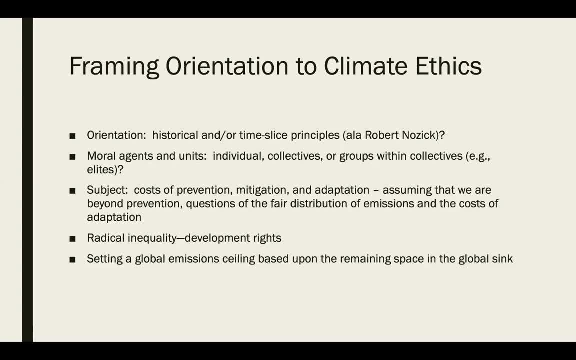 the fair distribution of emissions and the cost of adaptation are central to any climate ethics. what? what would constitute a fair distribution of the continued consumption of fossil fuels, for example, and who who should pay for the cost of adaptation? there's an argument from the developing world that the Western world 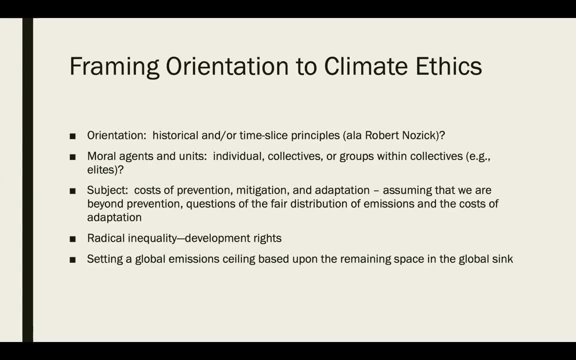 the United States, Canada, Japan, Europe. the Europeans have our response for for most of the climate pollution and have benefited the most from that from those emissions in terms of economic development, and the other parts of the world have been disadvantaged in their economic development and have barely contributed to climate change. why should they have? 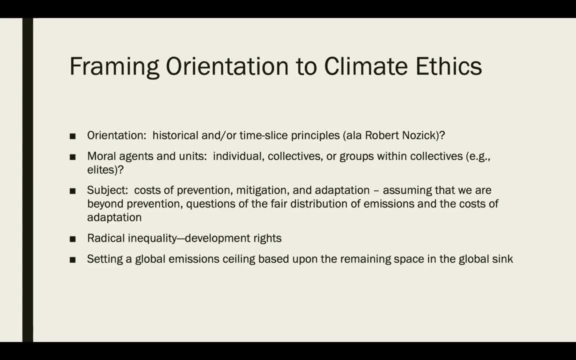 to bear, bear the cost, they argue, of the activity of European and American economic development. there's also consideration of, there's also consideration of setting a global emission ceiling based upon the remaining space in what is called the global sink. How much carbon can we, can the biosphere, absorb without? 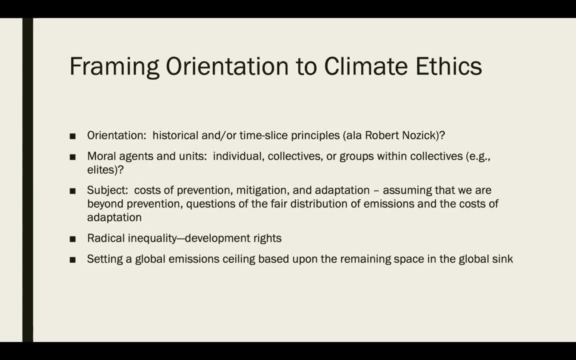 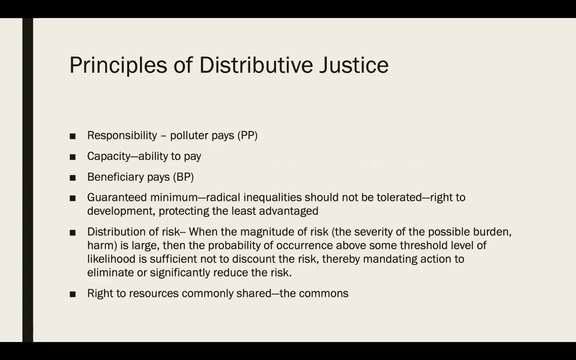 and how much can we sustain? how much carbon can we sustain in the atmosphere without very significant, and perhaps catastrophic, damage to the environment? So these are some of the issues involved in climate ethics and in terms of principles of distribution, of distributive justice related to climate. 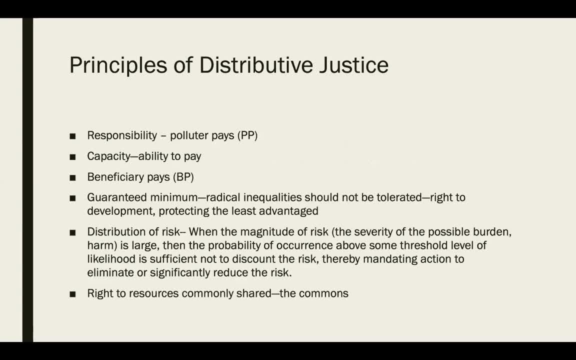 there's a number of possibilities: Capacity, responsibility, who's benefited? should there be a guaranteed minimum of consumption and emission? How should we distribute the risk of climate change? How concerned should we be about the consequences of climate change and the risk inherent in climate change? Could it be catastrophic? Are we willing to risk inaction? 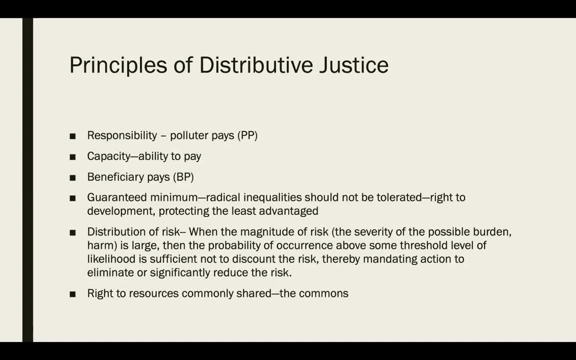 With the possibility of serious harm done to human beings and the planet itself. And who has the right to those resources? Is there? should we think of a commons? Is it fair that the United States, for example, makes up 4% of the world's population, but 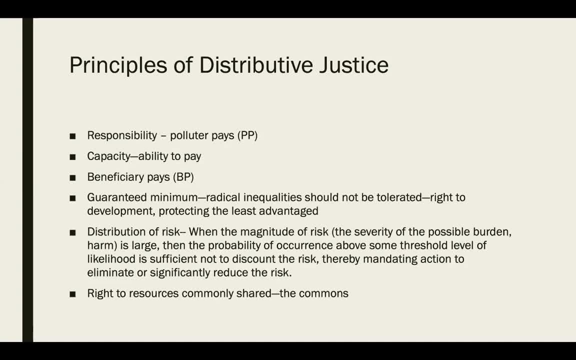 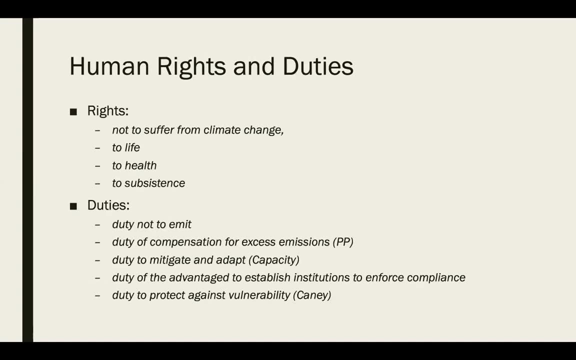 consumes 25% of the resources- Very high. Is that fair? Is that a fair distribution? So questions along those lines are important to in general, for environmental justice as well as for climate ethics. Dr Snower, may I ask a question? So do you think it's ethical for one country to produce a lot of humans? 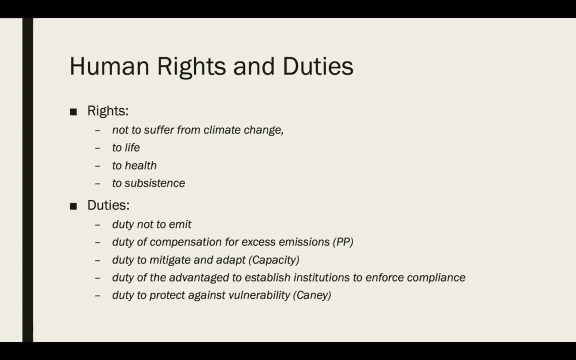 Well, that's a. that's an interesting. That's an interesting question. You mean you're talking about population control, Right? You know certain, like China- I mean, of course, we're the largest- So we did control, China did control, I would say we, but you know what I mean, no matter how long I live here. And so we- I mean China- did control the population, but that policy was so criticized. 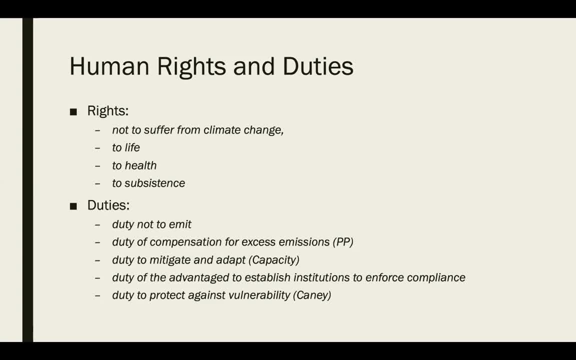 By controlling the population, China reduced the five, five million or something, whatever million, it's more than that, But now so is it not just China? in so many countries in the world they do not have birth control, So they have so many babies. is that ethical then? 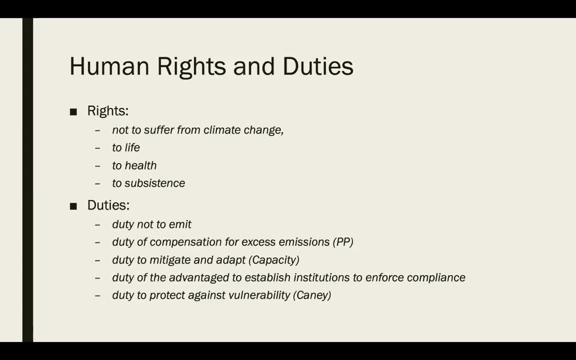 Because you consume more birth. Yeah well, I'm not sure if the ethical question is about the size of the population as such, but whether how we, what the population does in terms of the consumption of resources and the admission of pollution into the environment. 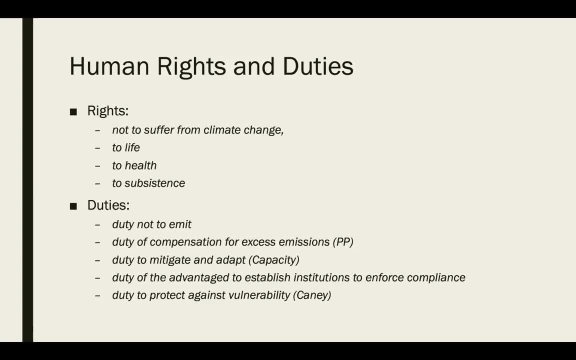 Population is a significant question but all projections suggest that the human population will level out at about 10 billion people and stabilize at about 10 billion And most of the increase in population to that level and leveling off of 10 billion will come from Africa. 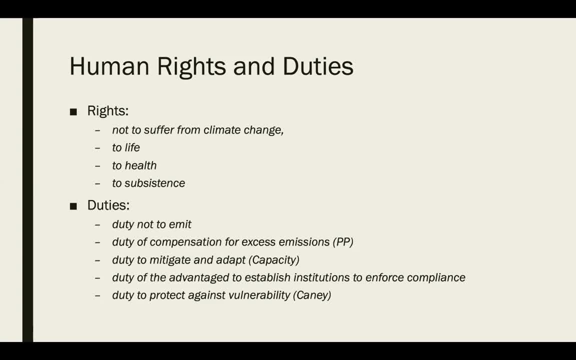 There'll be the African. Africa will be the center of future population growth going forward Right, so we'll have about two billion to go. Yeah, and it that's difficult, but there is hope and there is significant evidence, I think. 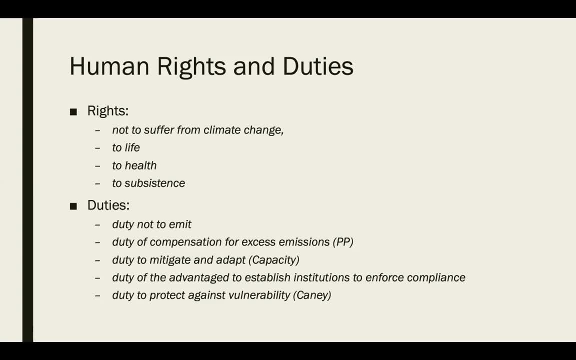 that the population will not grow beyond about 10 billion people. It's a lot of people and a lot of consumption, but we have to. given the size of the human population, we have to think about consumption patterns, our carbon footprint, our carbon economy. 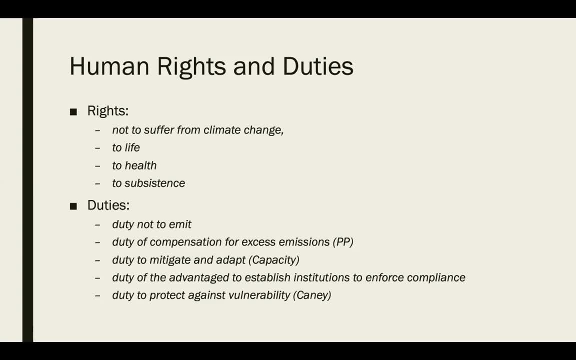 and how we can solve this. Yeah, that's a great point: footprint as a species and the development of other resources that are sustainable resources. So population growth was once alarming, but I think that has stabilized over time. It's more now a question of what we consume and what pollution we produce and can we. 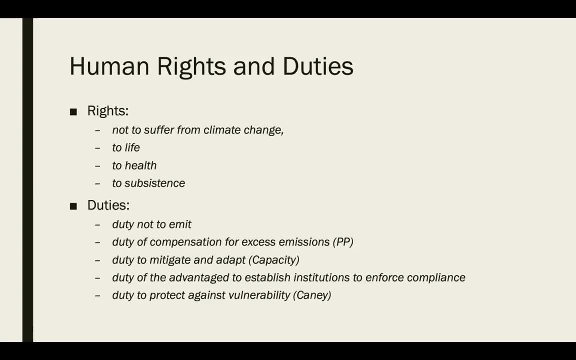 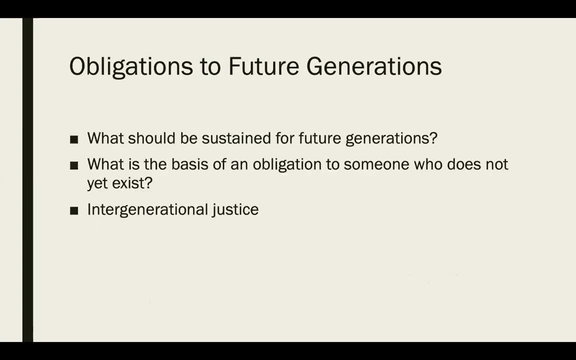 stay within the planetary boundaries of the biosphere. Okay, thank you. Another major consideration is intergenerational justice, that is, do we have obligations to future generations, And this is connected to both sustainability and climate ethics. Do we have obligations to future generations? 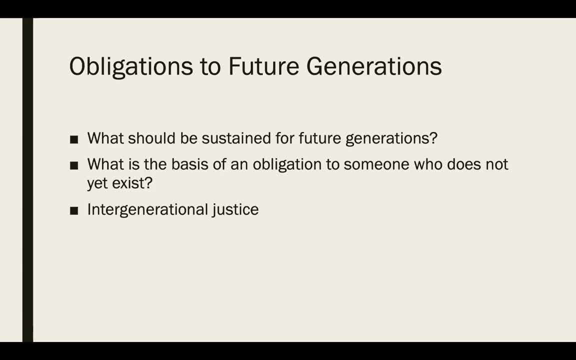 What is the basis of an obligation to someone who does not yet exist? And we could explore that. we will explore that further, But it's a fundamental question in environmental ethics: Is there an obligation, a duty, a moral duty to future generations of human beings as? 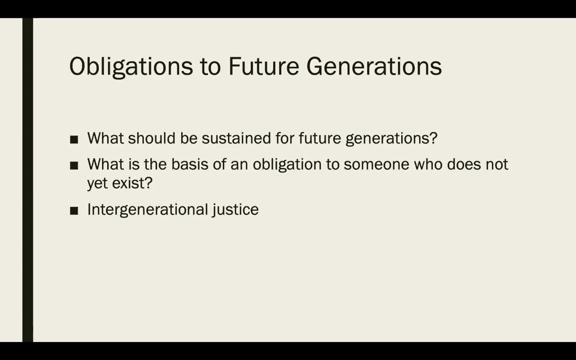 well as future generations of other living things. Do we have an obligation to the future? Many argue that we do. some argue that it's not possible to have an obligation to an entity or being who doesn't exist yet, But I think there are strong obligations. 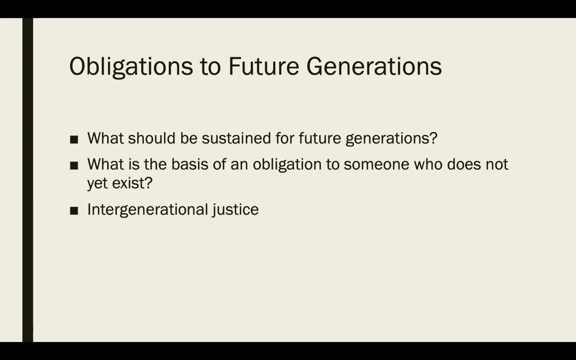 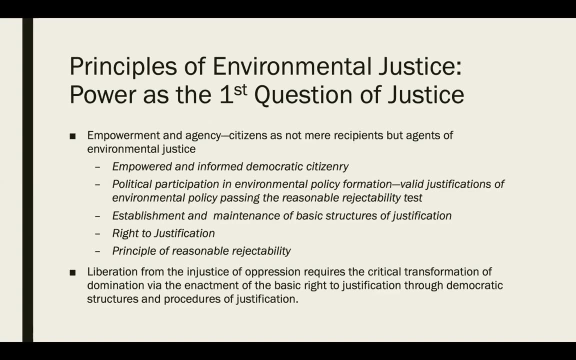 Thank you. Thank you Very strong counterarguments that would justify an obligation to consider, to give moral consideration to future generations. We can think of environmental justice as well, And this is something we might want to pursue further in the course. is the nature of environmental. 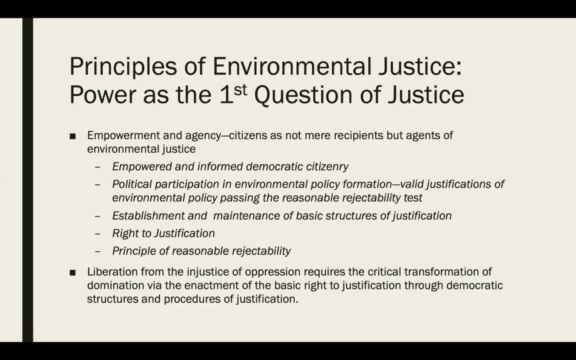 justice In terms of power and the empowerment and agencies of citizens as not the mere recipients but the agents of environmental justice. How do we empower, create an empowered and informed democratic citizenry who can participate in environmental policy formation? Thank you, 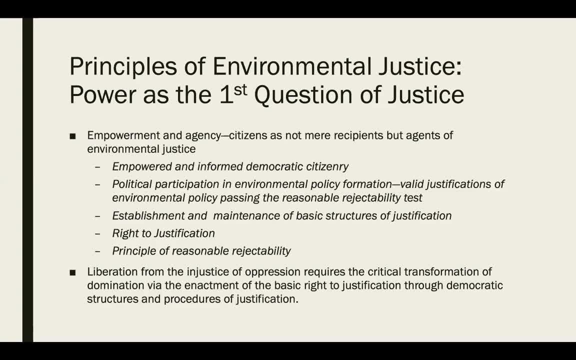 Thanks for the question. Thank you very much, Dr Lerner. So I think, as I've mentioned, the examples that are being made are still not the best. yet I think we're moving forward. We're going to have to do a lot of work already. 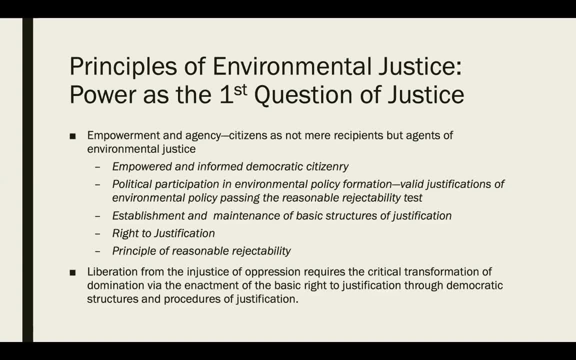 We're going to have to do a lot of work. We're going to have to do a lot of work. I think there's a lot of work to do, Yes, Yes, Yes, Yes, Yes, Yes, Yes- of the fair distribution of the rewards. 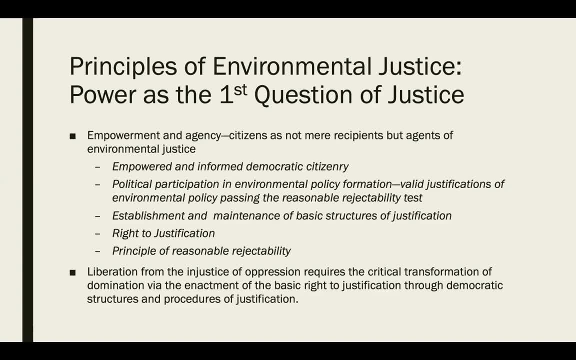 and burdens associated with environmental pollution. environmental sustainability. Often, historically, environmental pollution has been unfairly distributed to individuals of lower social classes. for example, which are sites of neighborhoods where poor people live are often more polluted and more toxic than environments where more affluent people live. 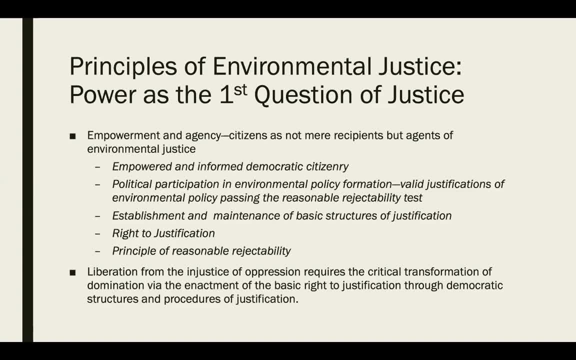 And when there's an interconnection between race, ethnicity, gender and income, then we have significant questions of environmental distributive justice which we can, we can consider going forward, And this relates back to the question of the fair distribution of environmental benefit. 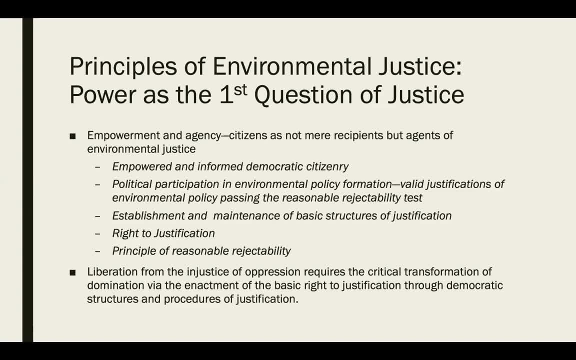 and environmental damage And who should share the burdens. How should the burdens be shared And how should the cost of creating an environmentally sustainable society, who should bear the burden, What are those costs And who should benefit from its existence? So questions of environmental justice. 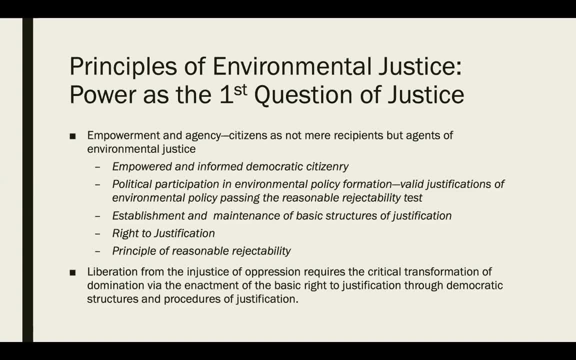 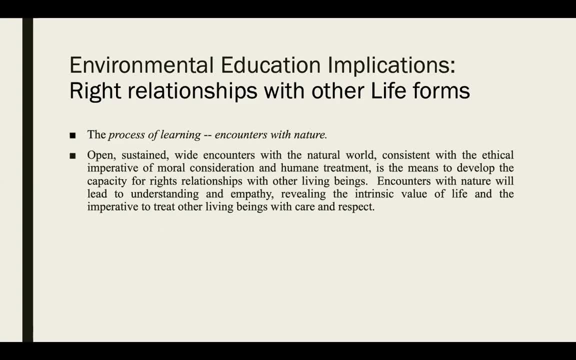 are also important, fundamental to environmental ethics. And then environmental education, the implications from an ethical analysis of our relationships with the environment. How can we conceive of an environmental education that would be environmentally ethical? One major consideration is, in terms of the process of learning that we have, educational approaches. 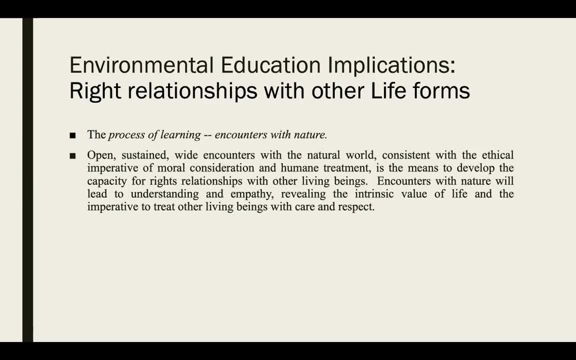 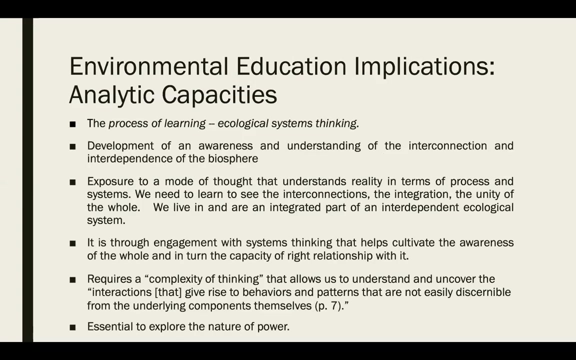 that foster encounters with nature that include the natural world, consistent with moral consideration And human treatment, to develop educationally, develop the capacity for right relationships with other living things, And so encounters with nature would be an important element of an environmental education, Also the development of certain capabilities. 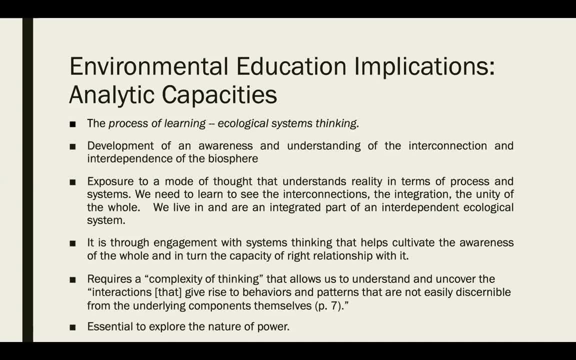 or capacities that environmental education would be, that would be devoted to, in particular, ecological systems thinking, the development of the awareness and understanding of the interdependence of the biosphere- Now we're interconnected- To cultivate the capacity to think in terms of process. 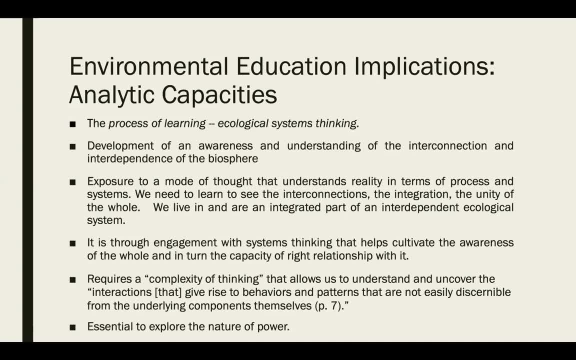 and integrated systems, to be able to concentrate on the process, to contemplate the interconnections of the ecological system, be an important capacity to develop and the development of systems. thinking that cultivates an awareness and the whole and a capacity to engage with that whole. 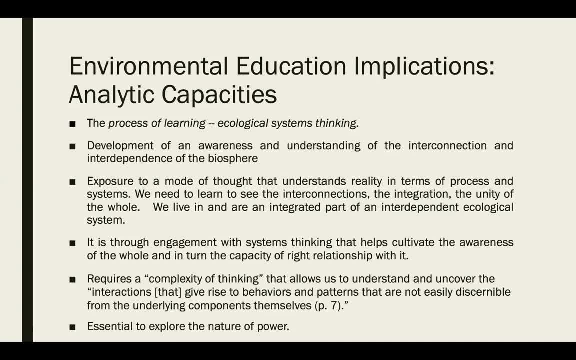 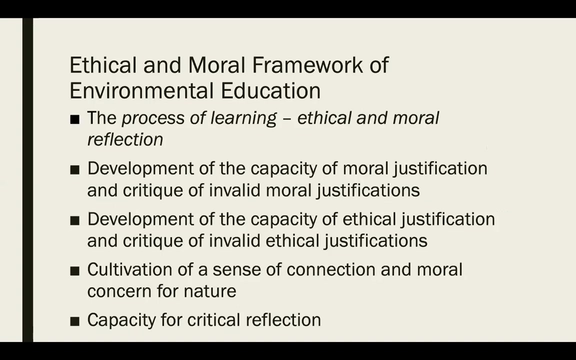 It also requires the capacity for complexity of thinking, to understand interactions and patterns that are discernible within our relationship with the natural world. And also it's essential to explore the nature of human power in relationship to each other and to the environment, And we would include in an environmental education.